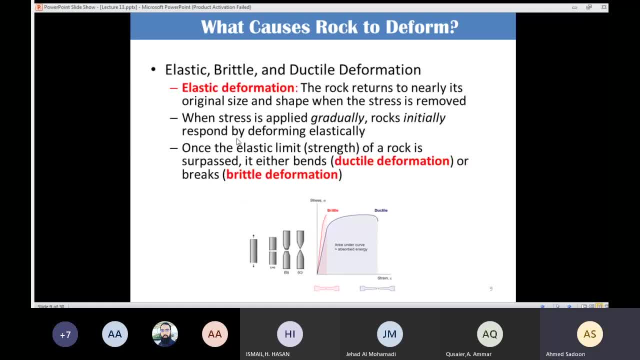 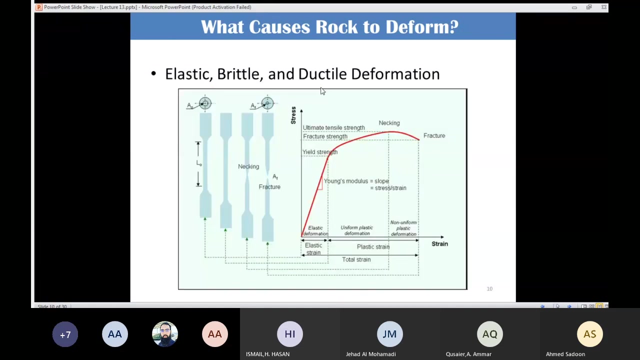 the tile deformation and I hope the idea is clear for you. it's very important concept. you are going to face that concept again and then again as long as you are in the field of civil engineering. so if you understood the elastic, brittle tactile deformation, the next courses is going to be easier for you. and we discussed also the factors that affecting 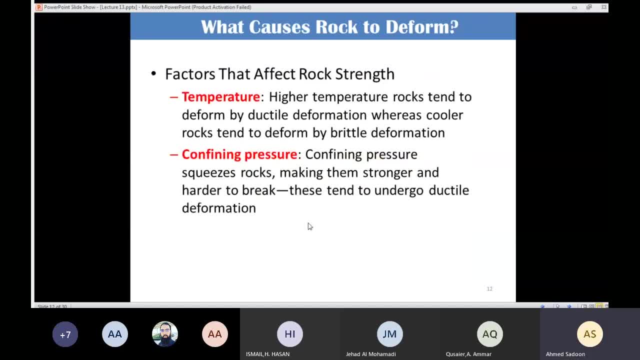 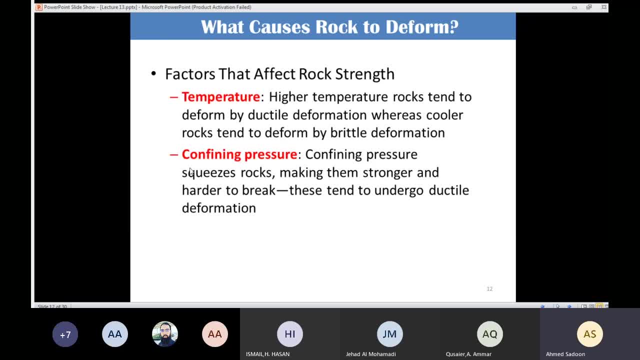 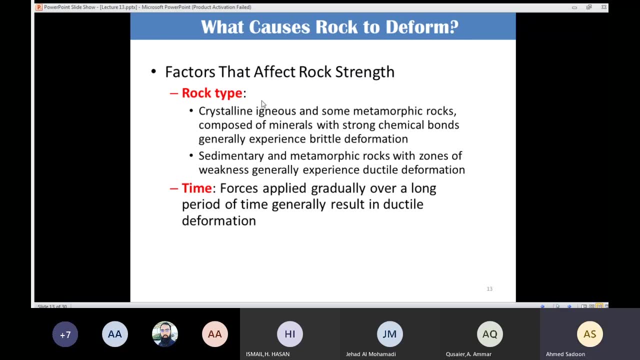 And also the effect of the confining pressure. If you have confining pressure, that means the rocks tend to undergo ductile deformation. And also we say that the rock type also it has effect on the ductile or the brittle behavior, as well as the time. 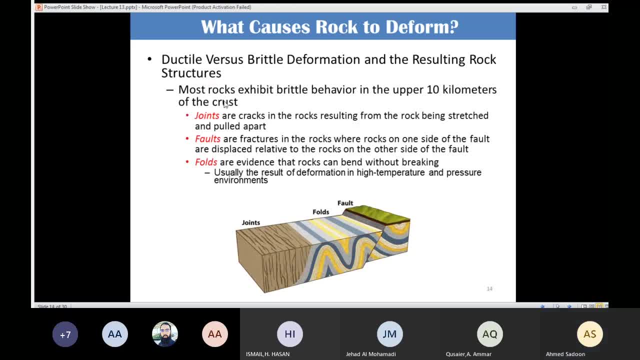 And we say that most rocks exhibit or show brittle behavior in the upper 10 kilometers of the crust And, as a result, you could have joints. This one is just like fracture And actually they are going to be parallel to each other without any relative displacement. 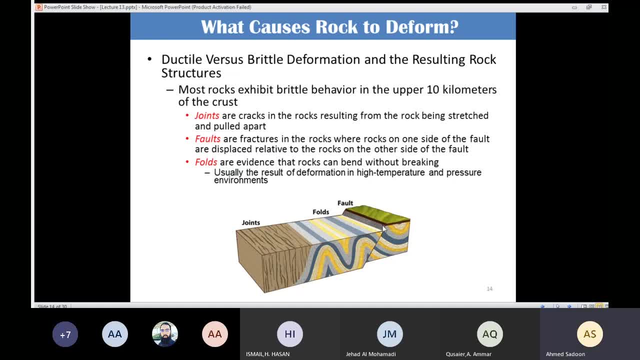 And we have the faults are going to have fracture like this one, But the fracture is going to be associated with relative displacement. Like you can see here, that part moved down relative to this part, And also we have the faults, which is like wave shapes. 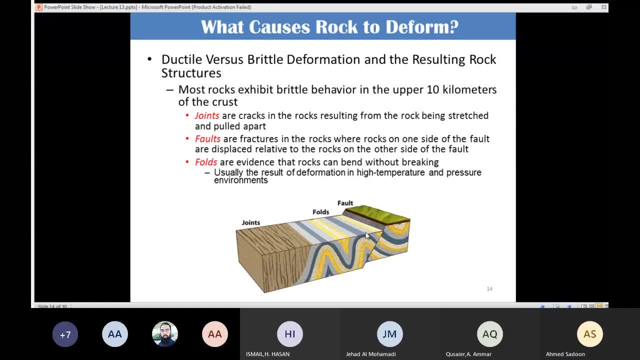 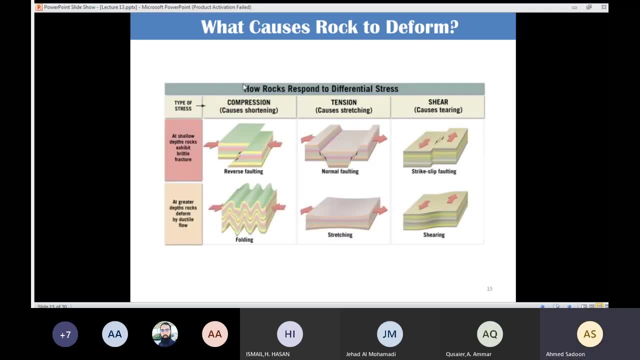 This is the wave shapes. This is the wave shapes. This is the formation: look like waves And mainly that because the rock is subjected to compressional stresses And the behavior is ductile. And here this table is important for you to understand. 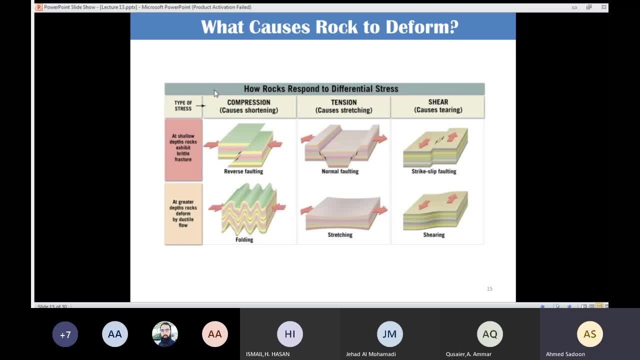 We have the columns. Column number one represent the compressional stresses. Column number two represent the compressional stresses. Column number three represent the tensional stresses And column number three represent the shear stresses. Row number one represent the brittle behavior. Row number two represent the ductile behavior. 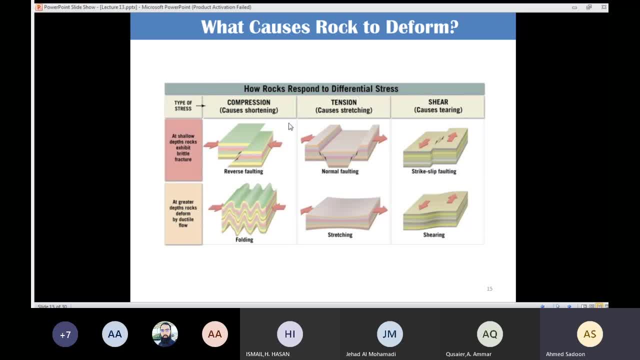 And, as you can see, you are going to have different types or different type of deformation. Although we discussed this last time, Today we are going to talk about the deformation. We are going to talk about the faults and the joints and the fault in greater details. 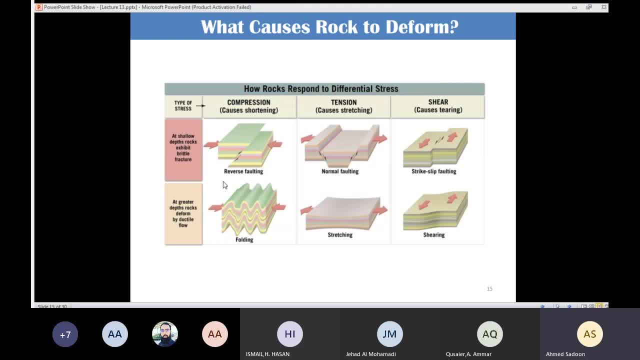 So we are going to start with the fault. Say that the fault, like you can see here, is going to form as a result of the compressional stresses And we need to have ductile behavior. So when I press the layer of the rock, I'm going to have wave shape, like deformation. 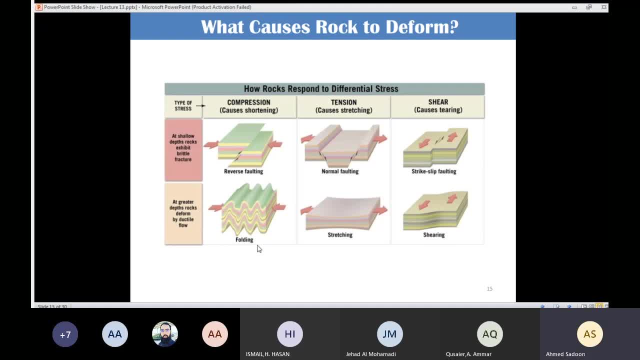 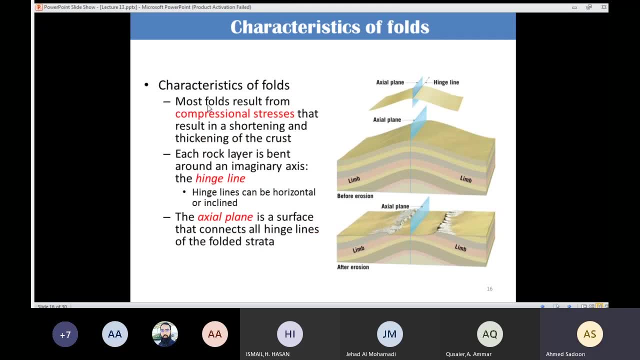 So if we are going to talk about the characteristics of faults, we need to know that most faults result from compressional stresses And because of that we are going to have shortening And thickening of the crust. So we are going to have shortening. 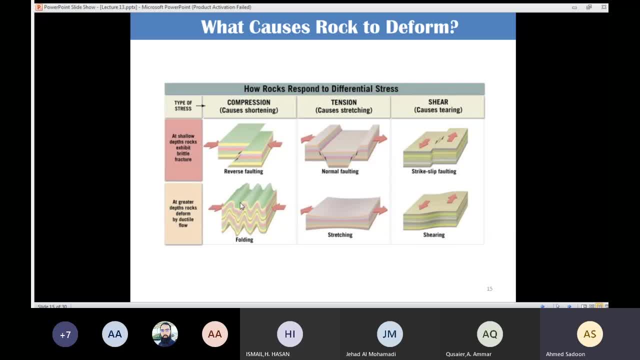 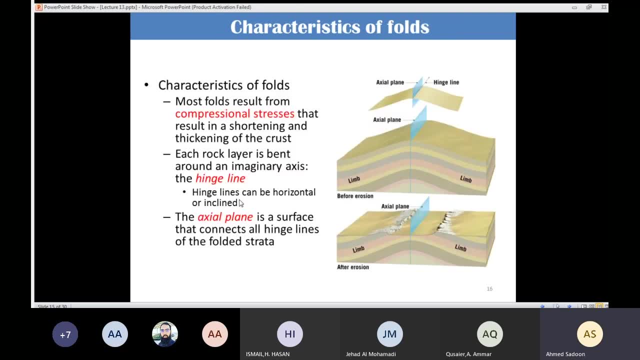 And the thickness of the crust is going to be increased, And there are some terms associated with the faults We need to understand. The first term is the hinge line. The second term is the hinge line, Because we are going to have waves like this one. 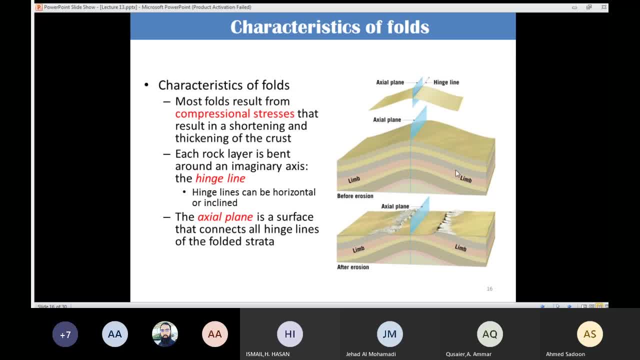 That means we have bending. So we have axis through which the limp, or the layers of the rock, is going to bend about. So the limp, here It's rotating about an axis. We are going to call that axis hinge line. So in this case, 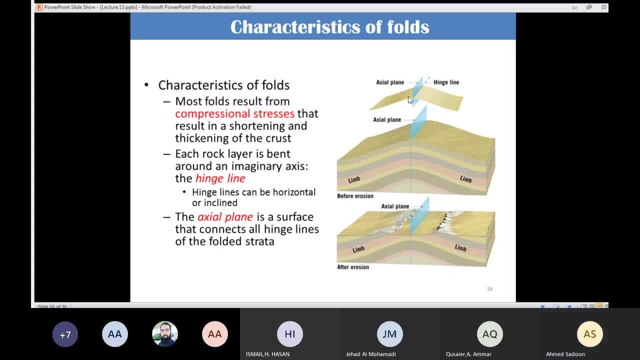 That line, here In that direction, Is the hinge line. It could be here, Or it could be here, Or it could be here. The most important point: The limp is going to rotate about That line. So Here is the hinge line. 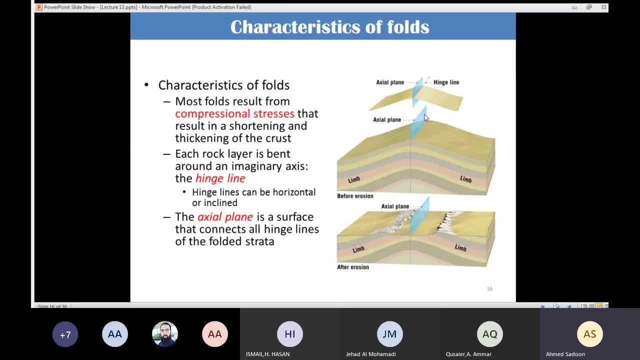 And if I am going to connect The hinge line, Assume this one, Hinge number one, Two, Three, Four, If I am going to connect them together, I am going to have a service, A plane service, And we are going to call it. 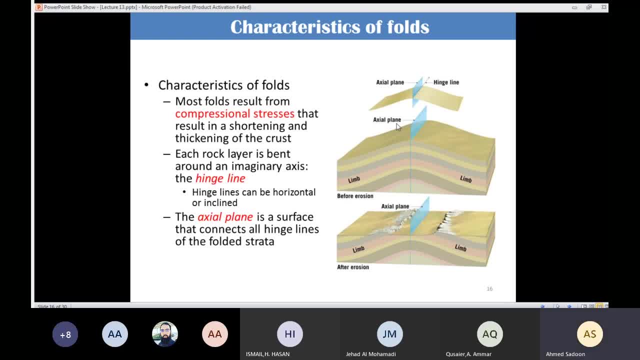 Axial plane. So we have Hinge line, Which is through which The limp is going to rotate, And we have the axial plane. It's a service, Connect all the hinge line And if you have Fold like this one, 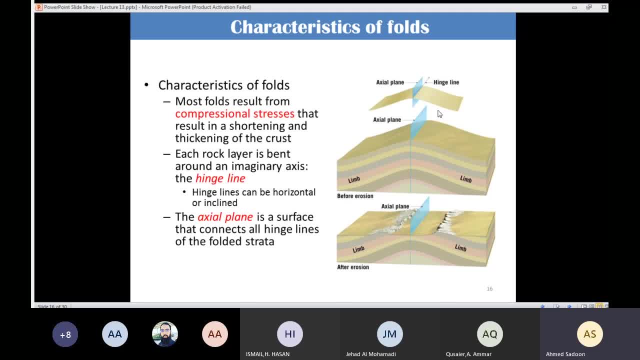 If it's subjected to Erosion condition, Because that part Is higher Than the other parts Here. This part is going to be eroded By the erosion Means Which we discussed earlier In the previous lectures. So 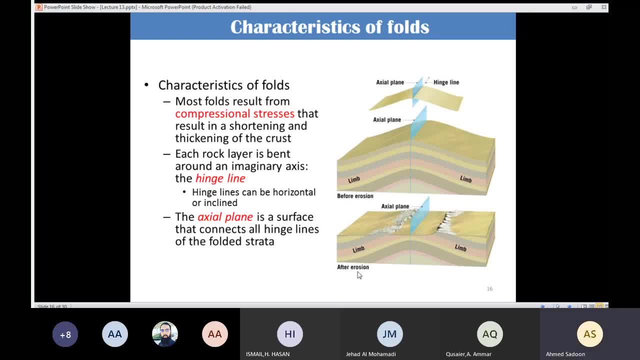 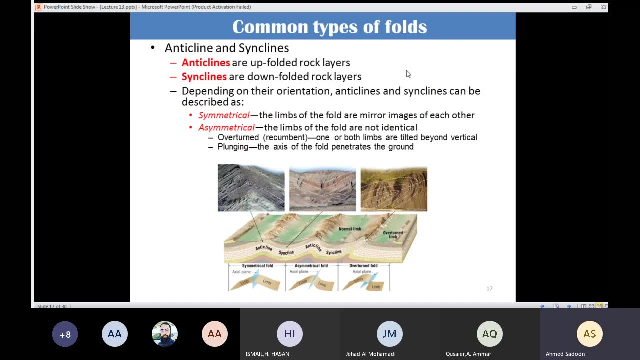 This figure here is before erosion And that figure here Is after the erosion And We have Features Or types Of the faults. If the faults Is going to be like that, In the wave shape We are going to, 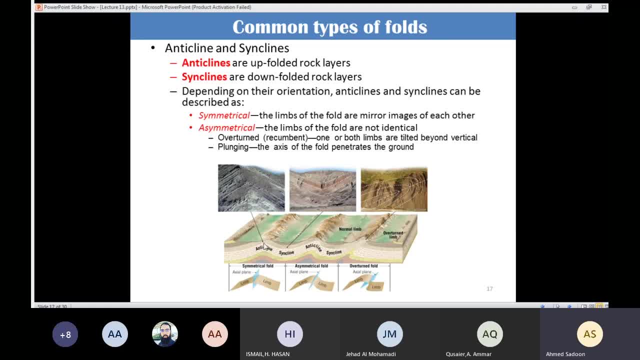 Call the up folded layer. Here we have Up folded layer And here we have down folded layer. The up folded layer We are going to call it Anti clients. So anti clients Refer to the Up folded Rock layers. 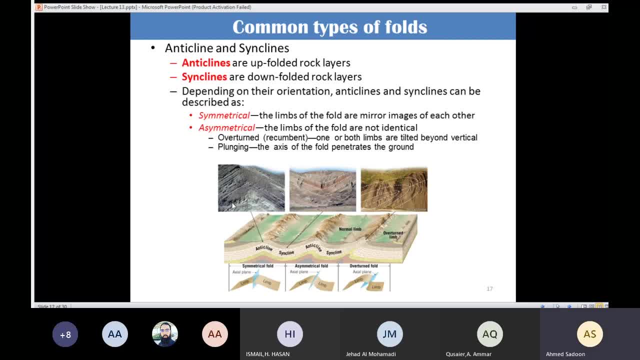 Like this one. So in reality, We are going to have something like that. So this Layer Is up, folded, Also this one, And that one Sink lines, On the other hand, Is opposite to Anti clients. This one: 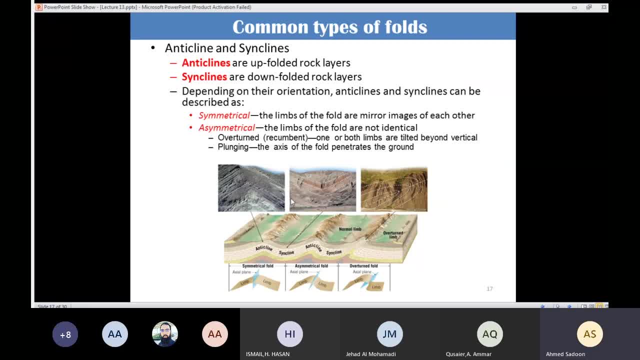 Sink line Is down folded Rock layers. In reality The layer It will be like that: Down folded, Like you can see here, So we could have Up folded Rock layers. We have Anti clients And we have 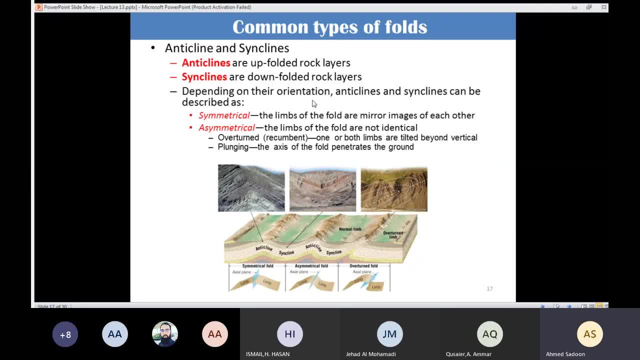 Sink lines And that depends On their orientations. The anti clients And sink lines Can be described as Symmetrical And asymmetrical. If it's symmetrical, That mean If you are looking at The axial plane, This part- 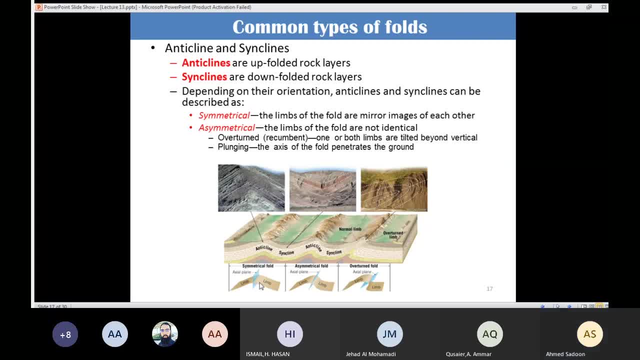 Is a mirror image For that part, Which mean, In other words, The limb On the left hand side Is identical to the limb On the right hand side. If it's Asymmetrical, That mean the limbs On the left hand side. 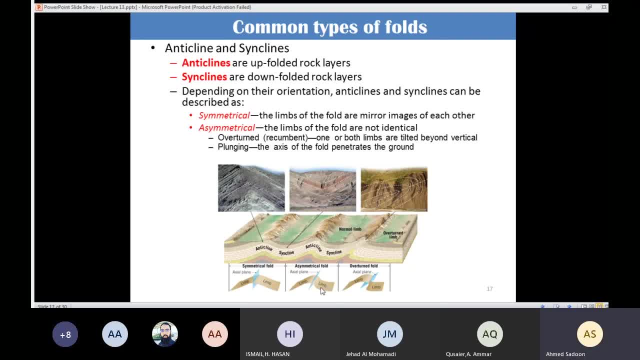 Is not identical to the limb On the right hand side Is asymmetrical fault, While this one Is symmetrical fault, The asymmetrical. Also, it could be Divided into Two types. We have overturn And we have plunging. 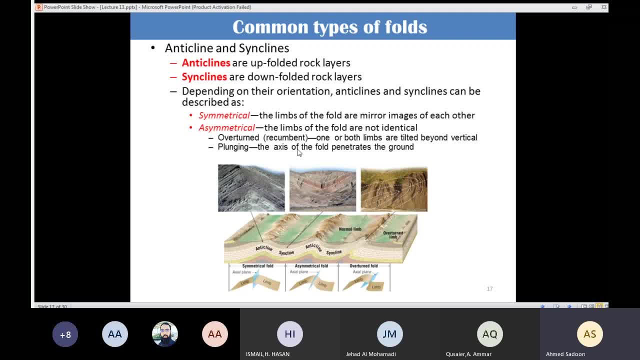 In the Overturn case We are going to have One or both limbs Are tilted beyond vertical, Like this one. If this one is a vertical one, We are going to have overturn. So this one Is a special case. 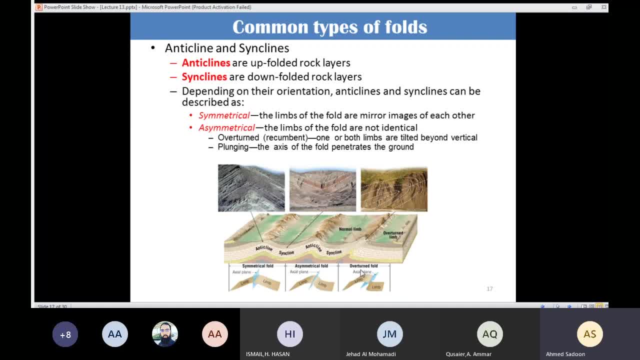 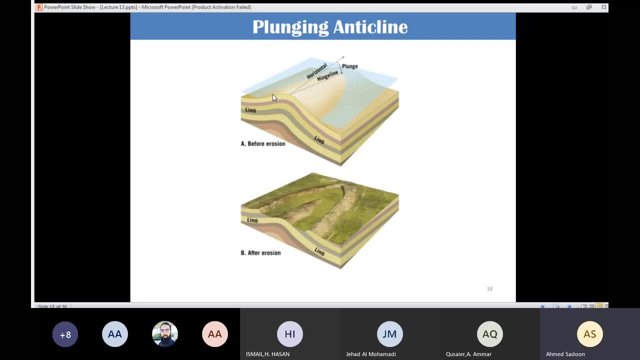 For the asymmetrical fault We are going to have Turning beyond vertical. The last case, Which is the plunging, Which is Like this one: here We are going to see that The hinge line, Or the axis of the fault, 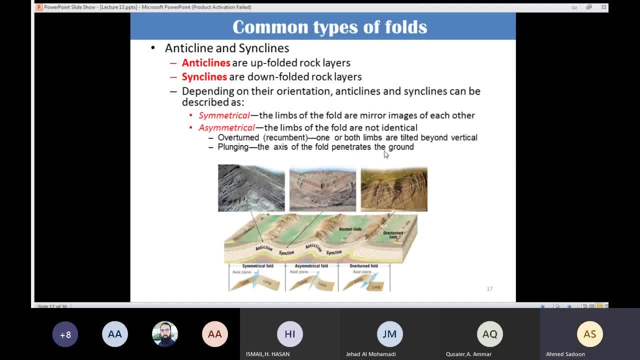 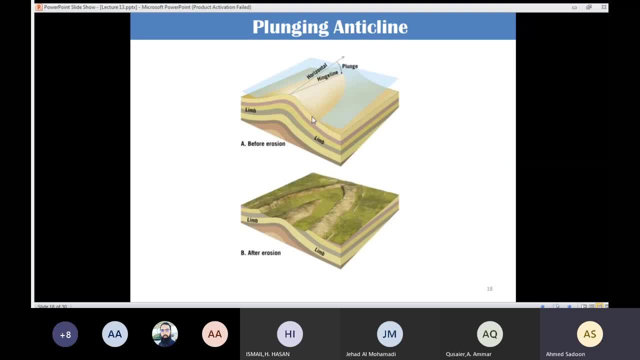 Penetrates the ground. So If you are looking here, If you are going to form A plane for that point Here, So we are going to form a plane Like this one And assume Here we draw horizontal line. 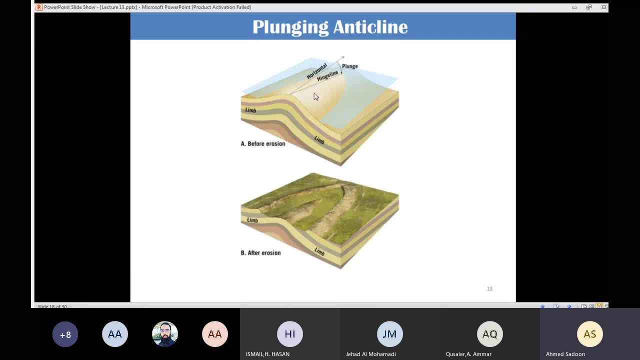 So if you draw horizontal line, That means I have displacement Between that line And that plane. It's going to equal that Distance here. And if you have Plunging and declines In that case The Axis of the fault. 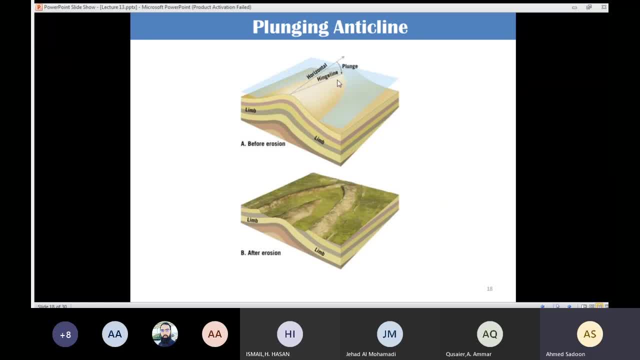 Is going to penetrate Inside that plane. So if you draw Angle here, We are going to call it Plunge angle- A value, Not zero, In other words The hinge line For that case Is going to penetrate. 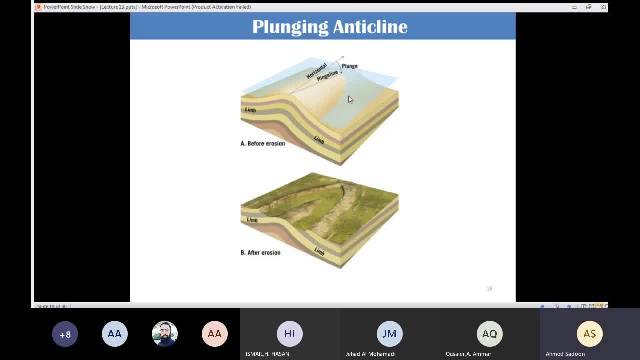 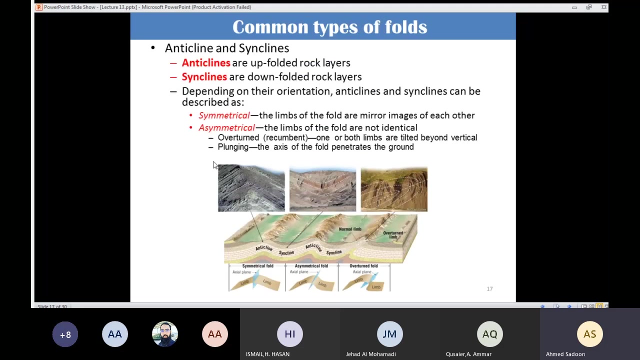 The ground, Which is this one, And If the erosion condition Are presented, In that case This part Is going to be Plunged. So We have anticlines, Which are The up folded rocks- This one: 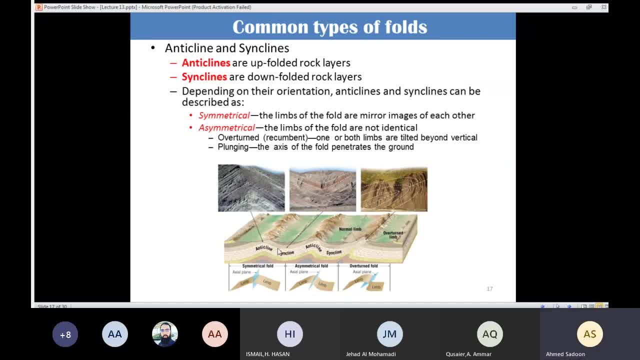 We have sink lines, Which is the down folded rock, And the anticlines Or the sink lines. It could be symmetrical Or it could be asymmetrical, And the asymmetrical It has special conditions. We have the overturn, Which means that 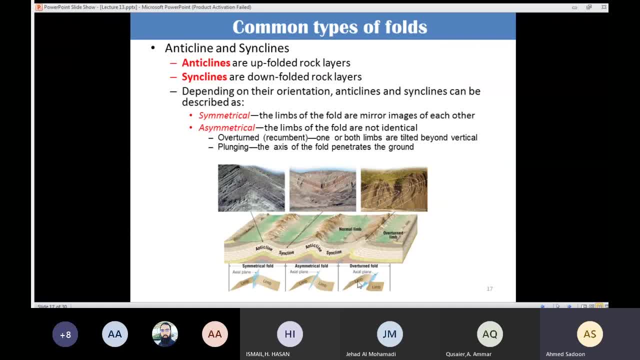 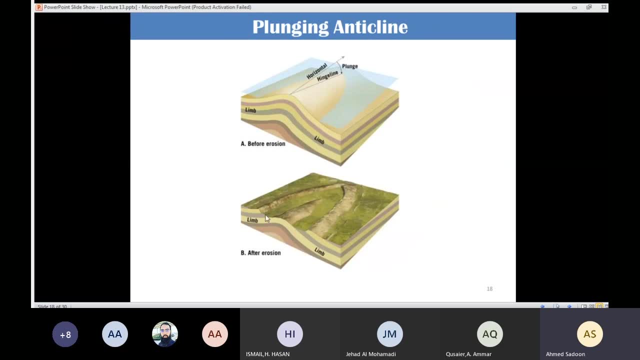 One or both the limbs Are turning Beyond vertical, While in plunging We are going to find that the axis of the fall Penetrates the ground, Like this case, And If we are going to have erosion, The figure is going to be like that. 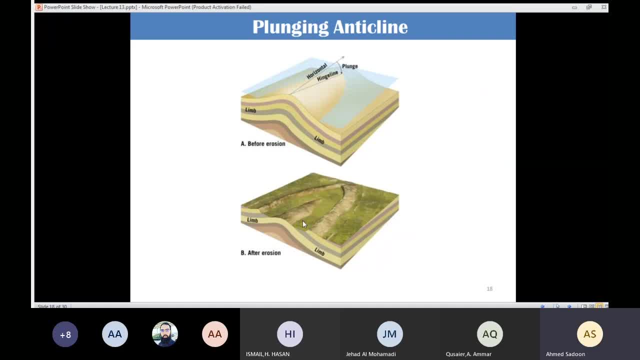 Any Questions? so far, Before we move on. I know here we have. We put a lot of information here. Okay, Be my guest. Excuse me, I didn't understand, Before erosion And after erosion, The figure here. 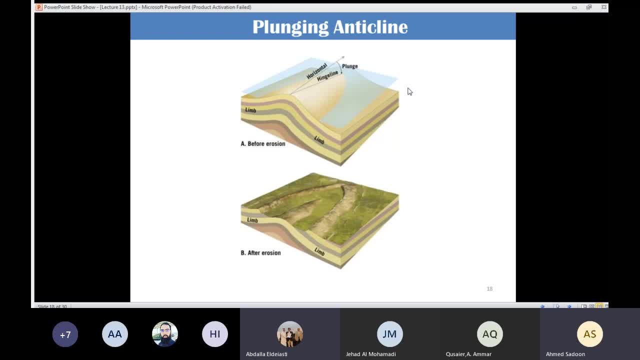 This figure here In front of me. After erosion, What happened to this Sectional area of the earth? We know that When you have a higher Plane here, Like this one, The wind Is going to be effective At that part. 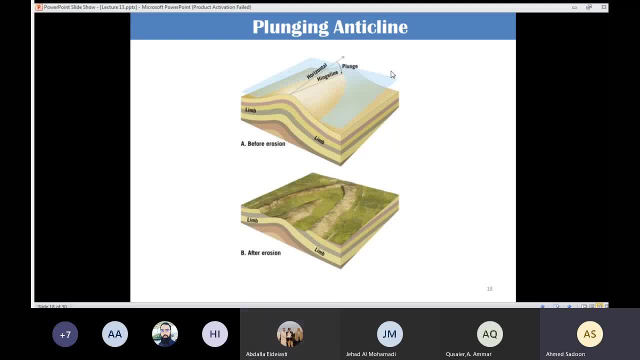 More than that part. Right, When a wind strike, Which one is going to be affected more, That part here Or that part? Of course, the top part. The top part Is going to be Subjected to The erosion conditions. 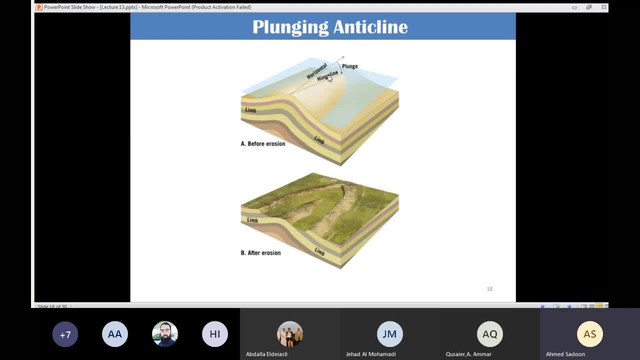 So we are going to say that If erosion are presented, In that case We are going to have something like that, Because the part here And some of the parts here Is going to be eroded And, as a result, I'm going to have something like that: 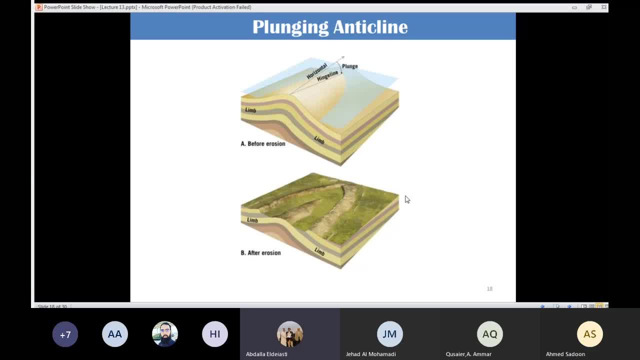 Hmm, Okay, The part in the middle, If the wind is, Is taking The top. Why did it take all of the top? The rest of The rest part Is it? It has the conditions, Which is just the natural. 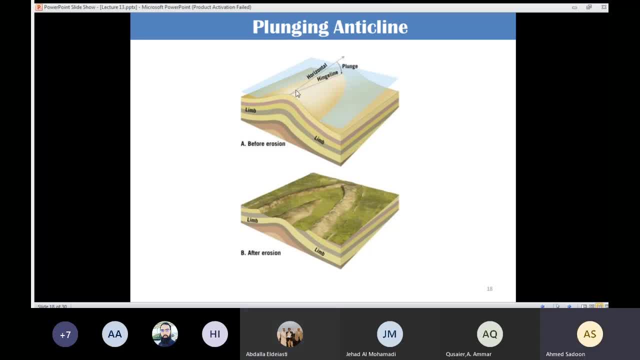 Think of this one like If you are going to have A knife Or going to have A knife, Then try to cut this one And try to see What will happen. Try to take a knife And take this part away. 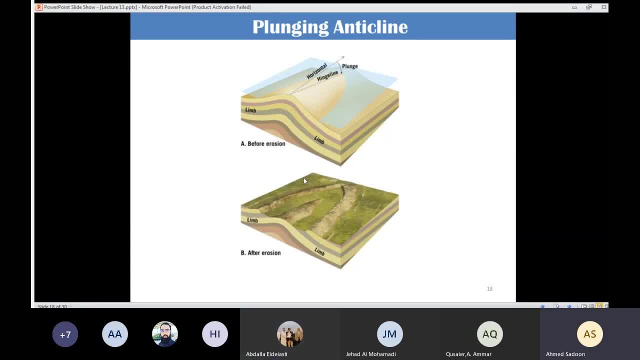 And try to look On the top side, You may going to Visualize The erosion, Hmm, But the main point is, If erosion take place, You are going to have Some other Types of faults, Like you can see here. 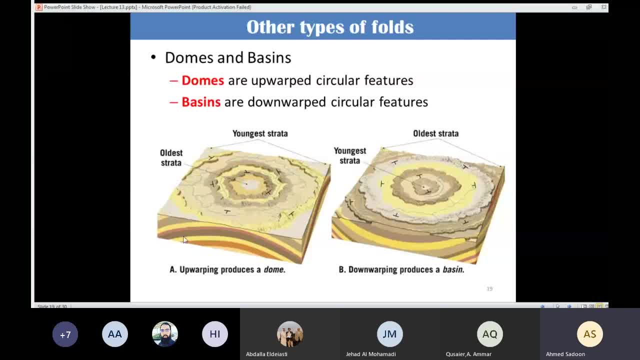 You have anticlines According to The layers. Here of the rock We have anticlines And Here we have Sinclines. So here we have anticlines And here we have Sinclines- Of course, Sinclines. 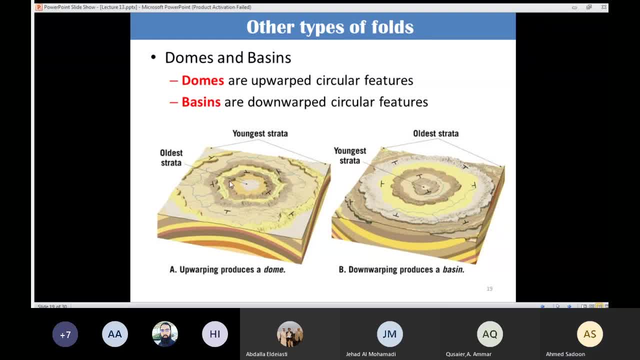 The layers here Is going to be the oldest Stratra And on the sides You are going to have the youngest Stratra, While in this case, Where you have Sinclines, The layers in the middle Is going to be youngest. 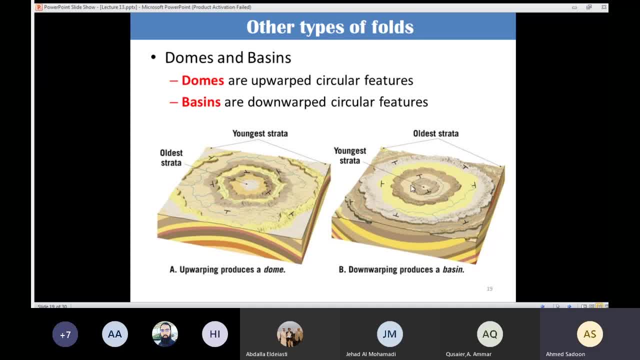 Stratra, While the one on the sides Is going to be the oldest Stratra, Because this one is Positioned in the higher places. The erosion Condition Is going to take the soil here And put it there, So this one is going to be. 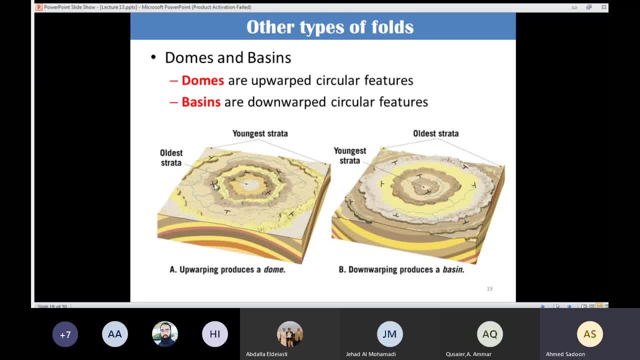 Youngest And this one is going to be Oldest. So this one represent the oldest Stratra And this one represent the youngest Stratra. And also, If you are going to have some conditions, Erosion conditions- 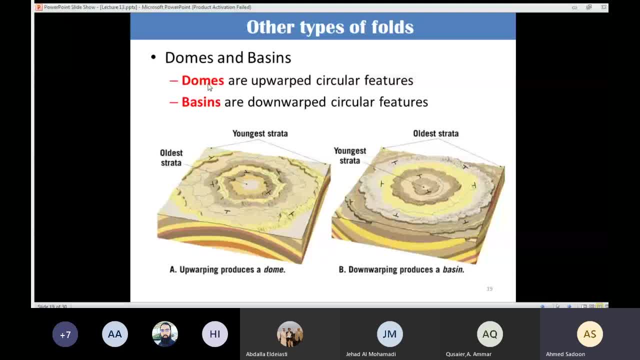 We are going to have Dooms In case of Anticlines And in case of Sinclines We are going to have basins. So we have the dooms, Which are described by Upwarded circular feature. 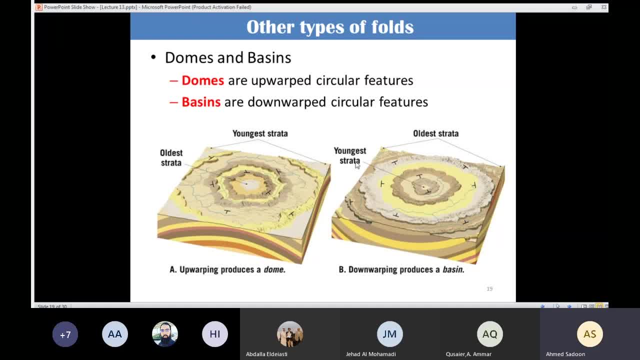 We have circular feature And in the basins Also we have Circular features, But this one is downward. Also is other type of defaults. The last one Is monoclines. The monoclines Is very large And it look like step. 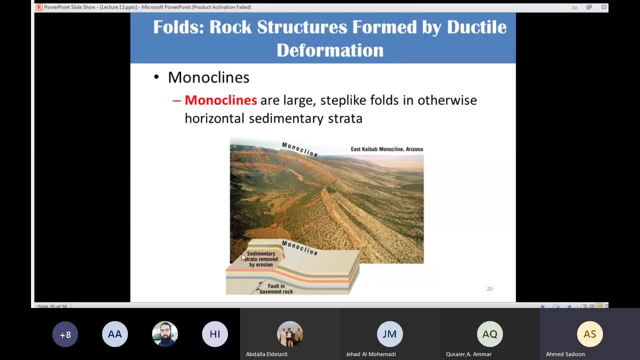 So Here The anticlines Look like step, Not like a wave. So If you have A large area- And this one Look like a step- And You have Horizontal sedimentary Stratra Like this one, 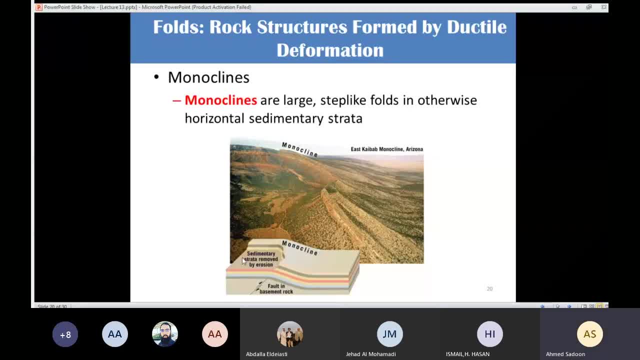 We call this monoclines, And if this one Is sedimentary stratra, It means that That part Is easily Removed by the Erosion. So If you are going to have Fault, But the fault In the shape of step, 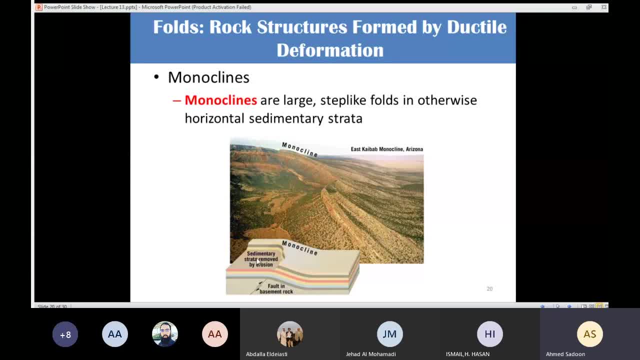 So this one Look like step And that part Is made from sedimentary rock Or sedimentary stratra, Then, As a result, We are going to have Something like that. So this one Is look like step And because this part 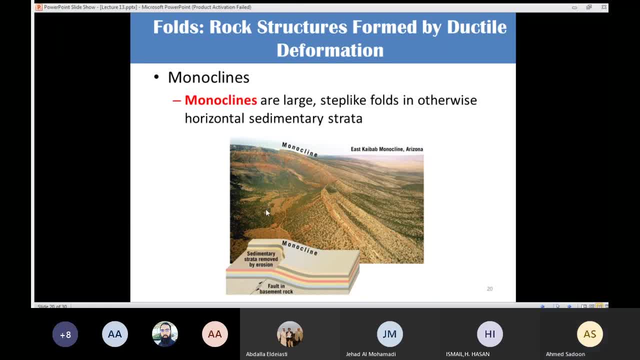 Is sedimentary stratra Is going to be removed by the Erosion And we are going to have Something like this one, Which is monocline. Any Questions about the type Of the faults? Okay, Let's move on. 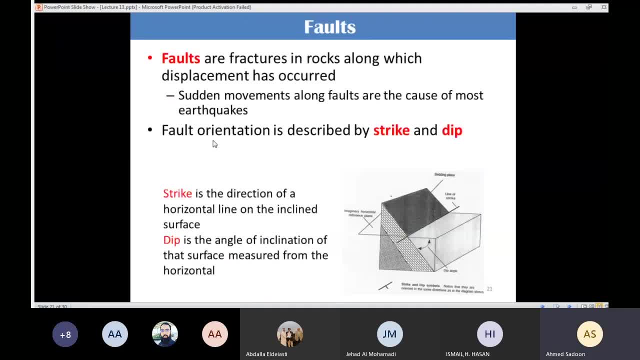 And We need to talk about the faults. And I want You to focus, Because If you missed small part, You are going to miss the other parts. So, please, I want you to focus here. We already defined the faults. 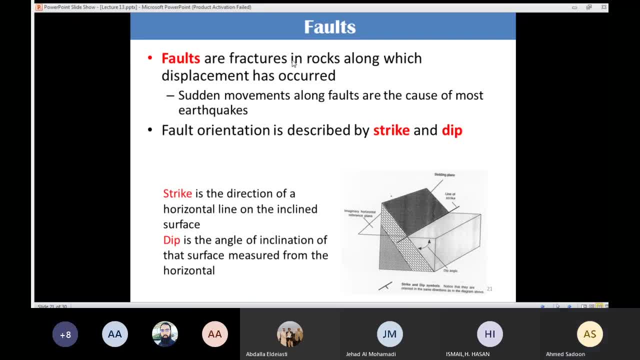 Say that The faults are Fractures. So If you have fractures- This one is rock number A And this one is rock number B And I have fracture between them- Then I have a fault, But This one should be associated with. 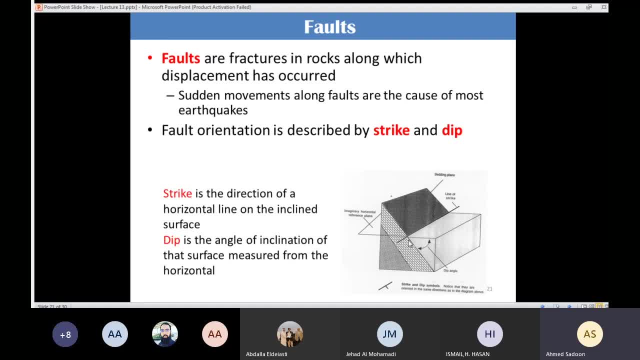 Displacement. So I need to have displacement Between rock A And rock B And that sudden movement, Displacement, Are The cause of the most Earthquakes And next lecture We are going to talk about the earthquake. 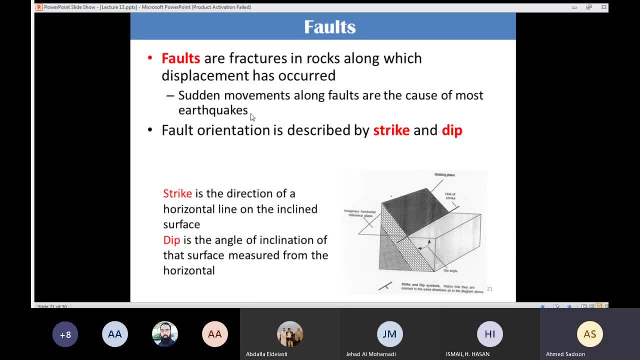 So Now we are going to have Strong, solid background Regarding the earthquake. So If you have a fault, The fault is going to be associated With displacement And in order To describe the fault, We need to know The strike and the dip. 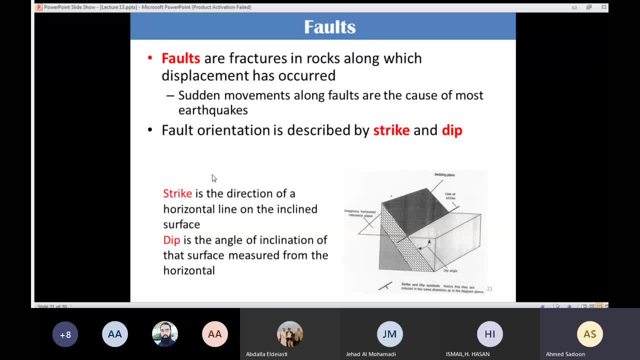 We have many types Of the fault And all of them are described by The strike and the dip. So very important to understand What does it mean by strike And what does it mean by the dip. So This one is rock A. 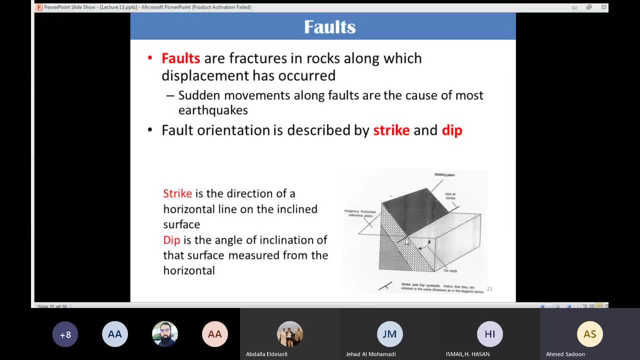 And this one is rock B And the fault is going to take place here And it is going to be associated With displacement: The direction Of the horizontal line On the inclined surface. This Is the inclined surface And here we have the 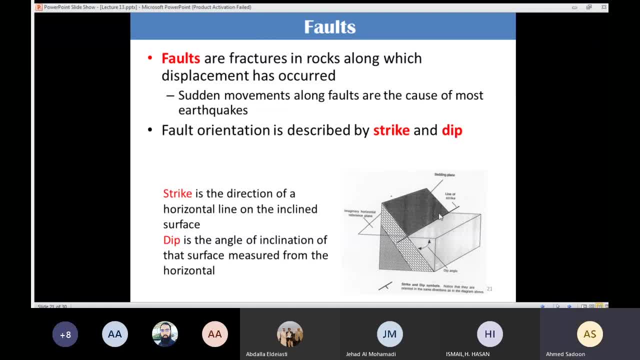 Horizontal line. So We call this strike Or line of the strike, And the dip Is the angle Of inclination. So the dip Is the angle of inclination Measured from the horizontal surface. So I have the strike, Which is the horizontal line. 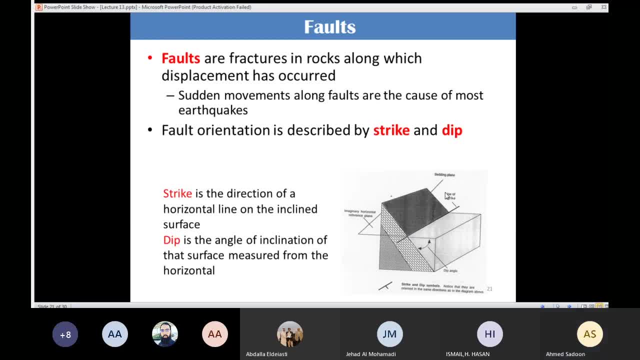 On the inclined surface. So if you draw a horizontal line On that inclined surface, We are going to call this strike, Whereas That angle here, The angle of inclination Which is measured From the horizontal surface, We are going to call it. 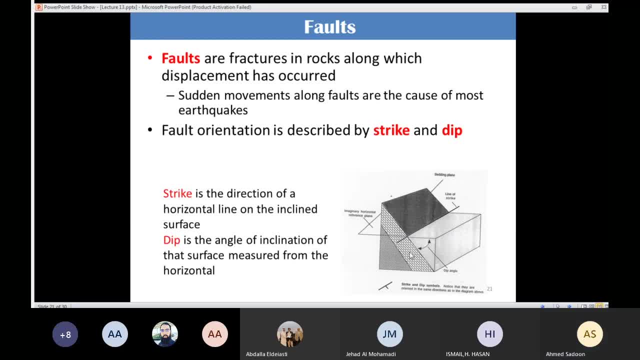 The dip angle. So We have the strike And we have the dip. We are going to describe All types of the faults By their strike Or by their dip. So Any Questions about the strike And the dip? 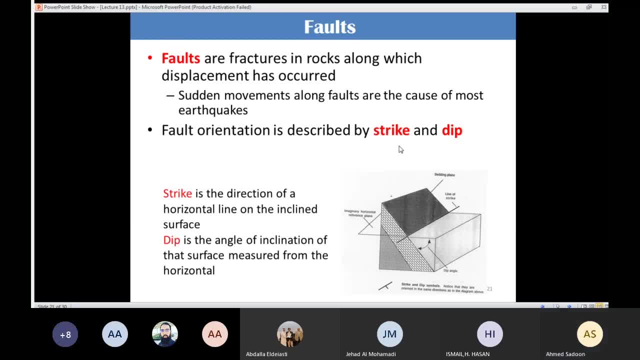 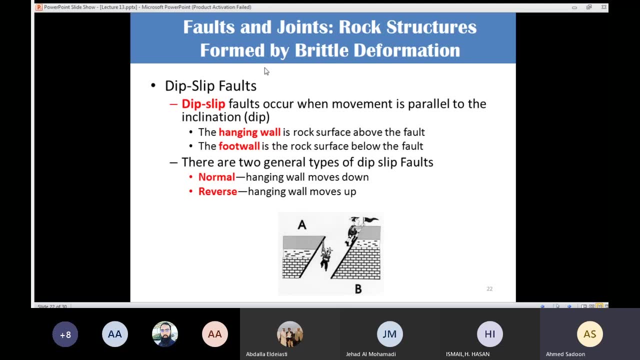 It is very important To understand this: The strike and the dip. Okay, So the first type Of the dip Slip, The first type of the faults, We are going to call it Dip slip, Slip means displacement. So in this type of the fault, 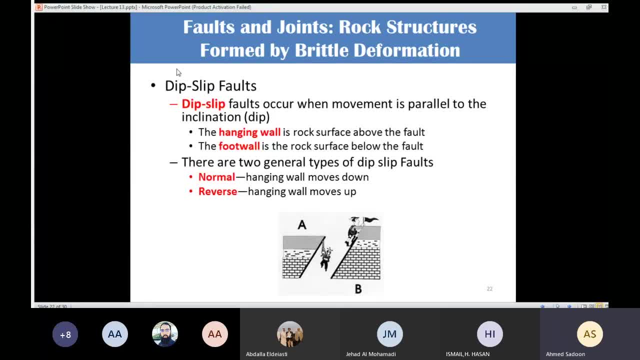 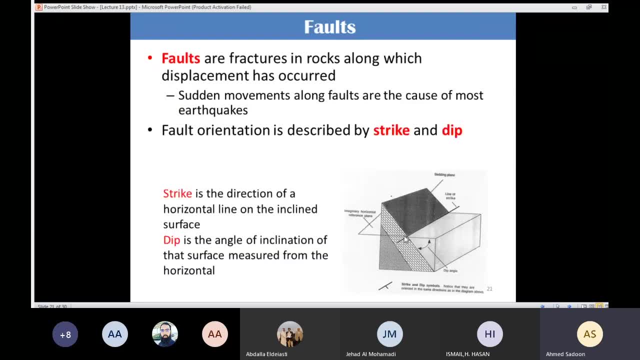 We are going to have Displacement In the dip, So this one is the dip. We are going to call this Dip direction And in this case We are going to have displacement In the direction of the dip. So 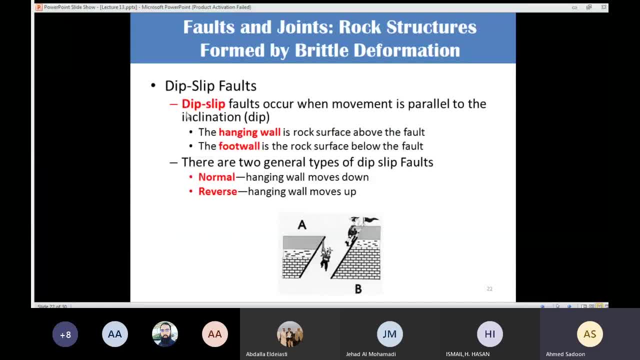 This type. here It has been described By the dip And we are going to call it Dip slip. So this one is the faults When movement is parallel To the inclination Or the dip. So here we have inclination, We have the direction of the dip. 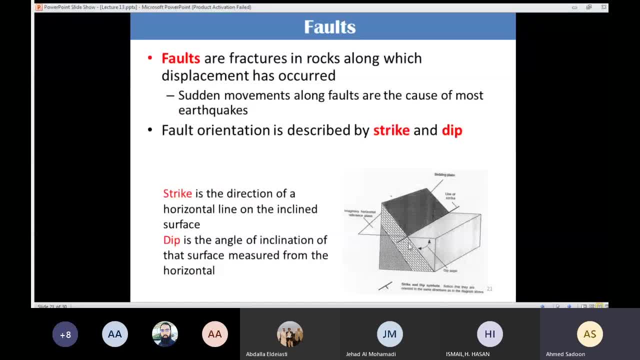 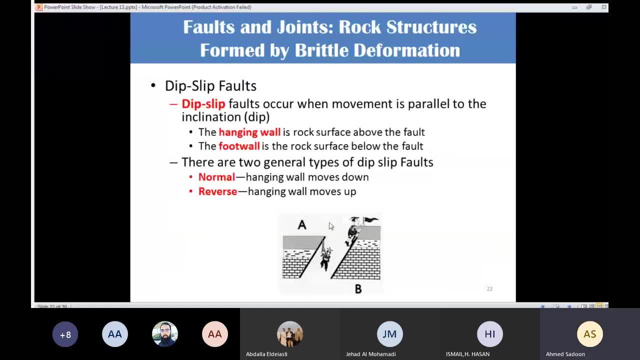 We are going to have Displacement or movement Parallel to the dip And Again We need to understand Very crucial Or crucial idea, Which is the hanging wall And the foot wall. So Assume you are sitting here, 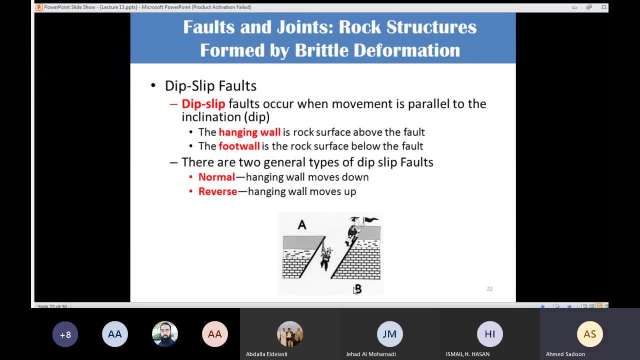 And Rock A and rock B Was A one unit And you were sitting here. Then Part B or part A, Spread it From part B And you are sitting here And you are Going, Or if you are planning. 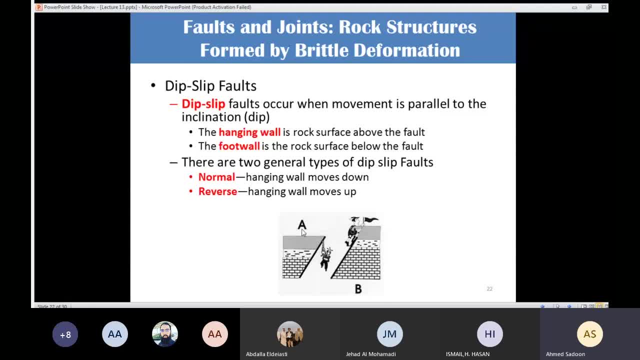 To go To the service of the rock A. In that case, You are going to hang yourself In order to get here. Then What if I am go? What if I want to go To the service of the rock B? 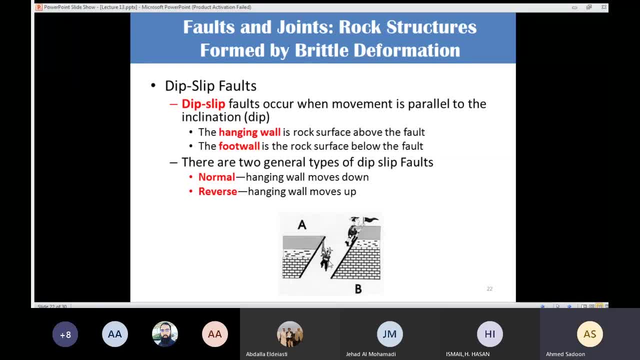 In that case, I am going to use my Feet in order To go there, The rock On the right hand side. We are going to call it The hanging wall, Because I need to hang Something In order to get there. 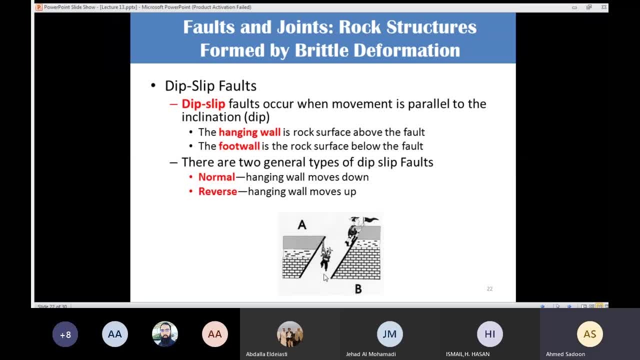 While the rock On the right hand side, This one. I need to use my feet In order to get there, So I am going to call this Foot wall block. So this one is the foot wall block And that one is the. 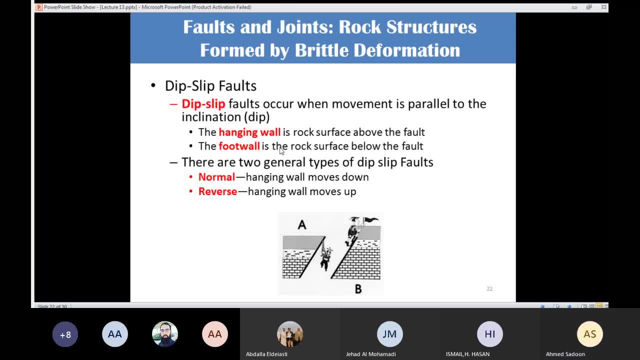 Hanging wall block And the hanging wall Is the rock service Above the fault. So the rock service here Is above the fault, While the other one, The foot wall, Is the rock service below the fault. So It is very important. 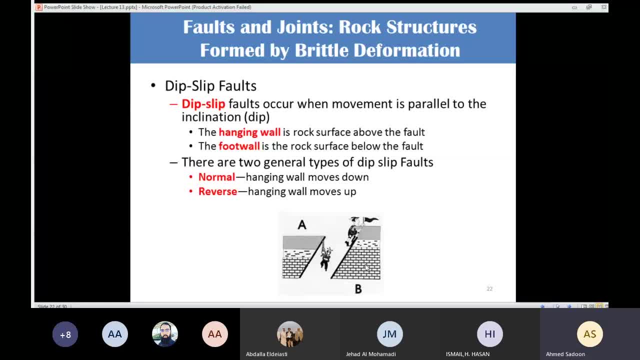 To differentiate between The hanging wall And the foot wall And the deep slip Which is described by It's deep, The direction of inclination. We have Two general types Of deep slip fault: We have the normal And we have the reverse. 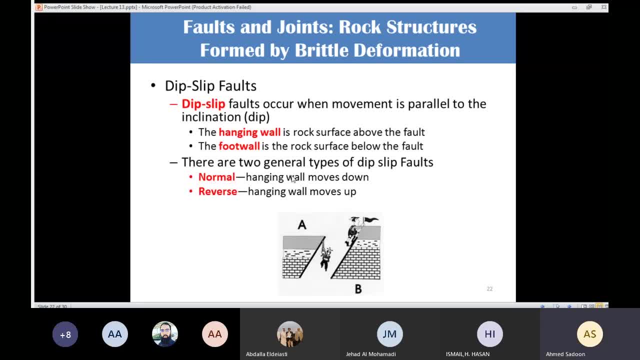 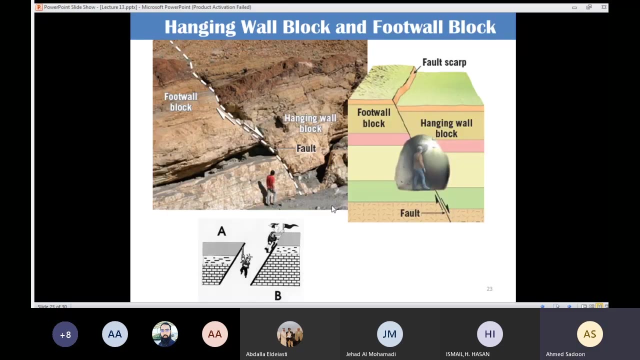 If it's normal, Then the hanging wall Moves down. The hanging wall Is going to move down. If it's reversal, In that case The hanging wall Is going to move up. So again, If you are Stuck here, 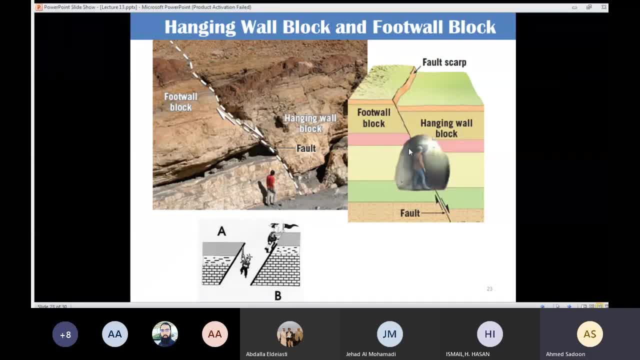 You should be able To know Which one is going to be the hanging wall And which one Is going to be the foot wall block. If I'm sitting here, If I'm going to Go to the Service of that rock here, 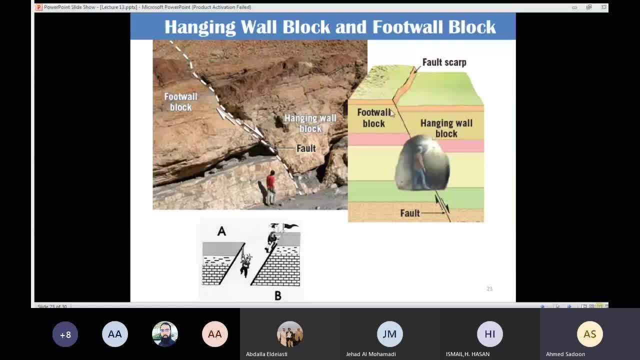 I need to hang something, Hang a rock In order to help me to get there, Whereas if I want to Get to the service of that rock, I need to use my feet. So this one is the foot wall block And this one is the hanging wall block. 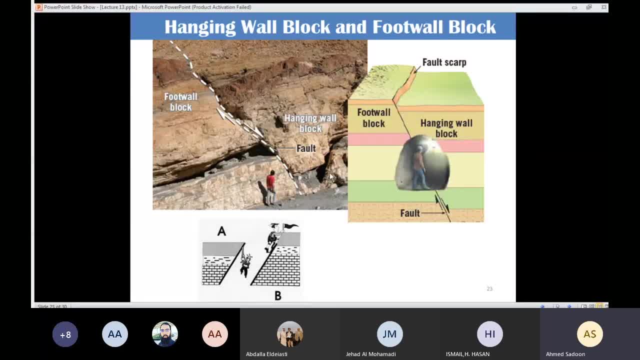 And here I have that case. I have deep slip And I say that It could be normal Or it could be reverse. If it's normal, That means the hanging wall Is going to move down. If it's reverse, 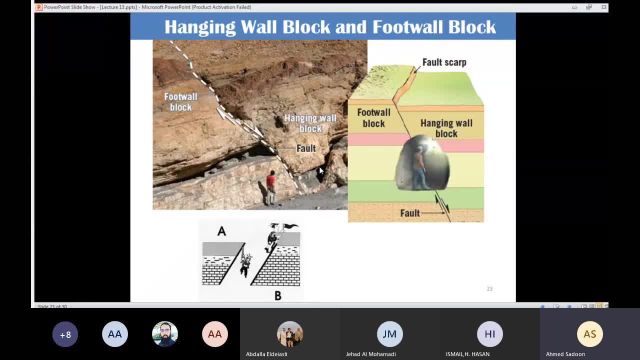 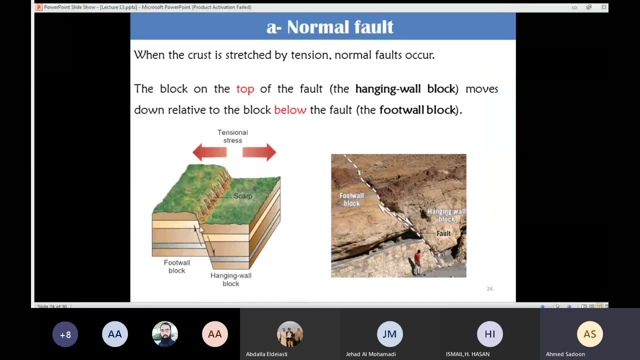 It means The hanging wall block is going to move up. So Here we have the normal fault. So If I'm sitting here, So I need to hang something, It means this one is the hanging wall If I'm here. 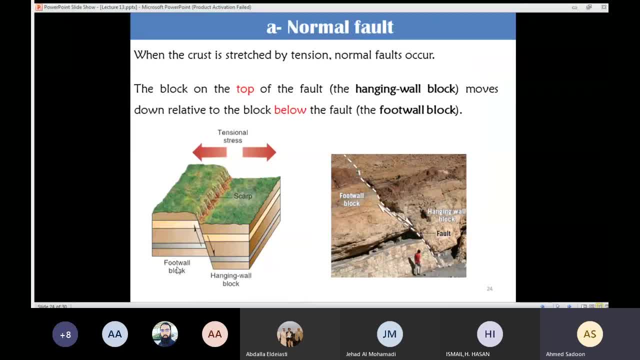 I need to use my feet in order to get there And this one as a result. This one is the foot wall block And here we have Movement. So obviously This one Is down. It means that I'm going to have 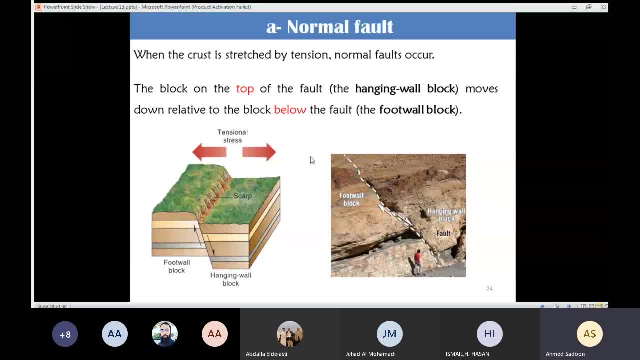 A normal fault And also the normal fault Is associated with the tensional Stresses. So the first condition For the normal fault, I need to have tensional stresses And the other condition is The hanging wall Is going to move down. 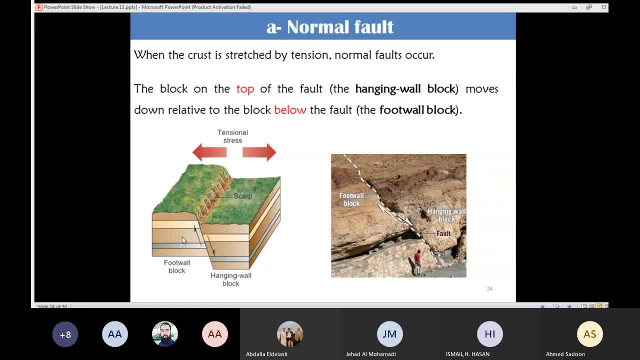 Relative to the Foot wall block. Here we have real picture for that. As you can see here That layer- It should be there- Which means that I have relative movement Of the hanging wall Relative to the Foot wall block. 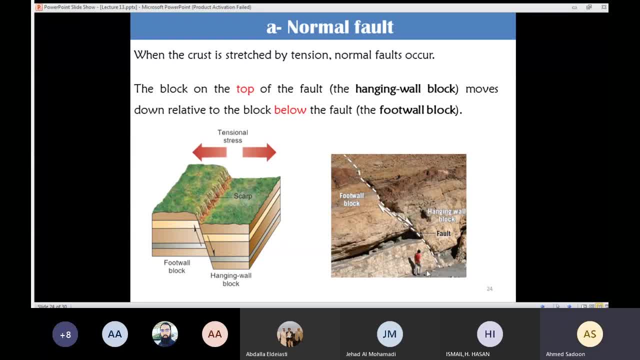 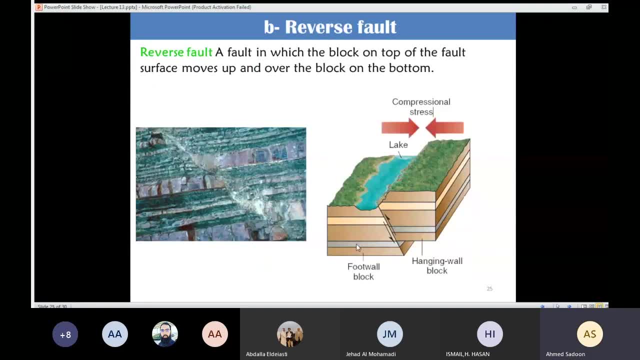 Which means that In that figure, I'm witnessing Normal fault. The other one, Which is the reverse fault, Instead of having Tentional stresses, In that case I'm going to have Compressional stresses And in that case, 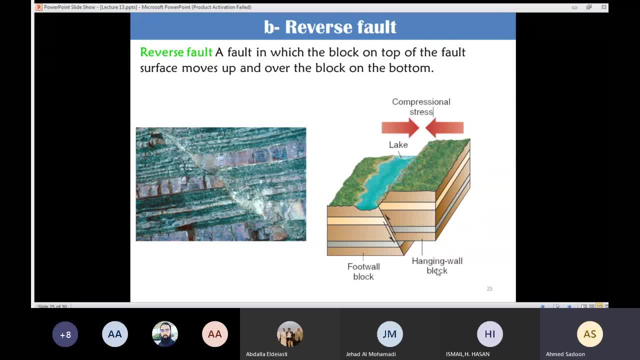 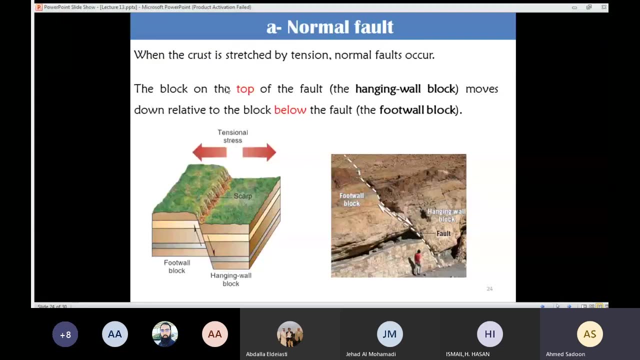 The hanging wall block Is going to move up Relative to the Foot wall block. So this one is a normal fault And this one is the reverse fault In the normal fault. I'm going to have Tentional stresses. 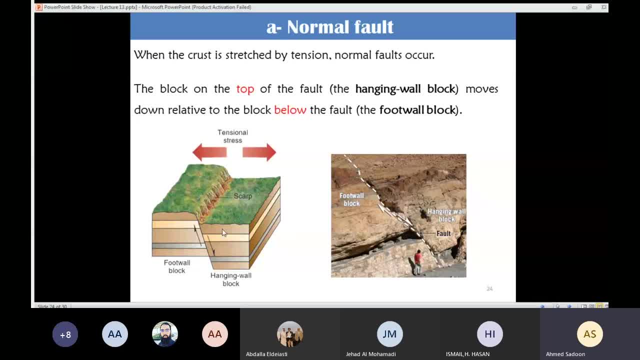 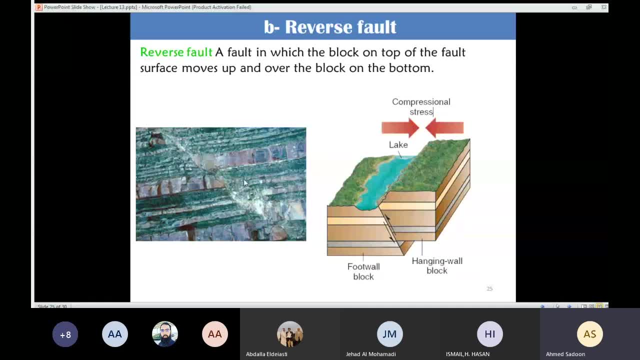 And the hanging wall Is going to move down. Here I'm going to have Compressional stresses And the hanging wall block Is going to move up. Like you can see here, This part and this part Were one unit. 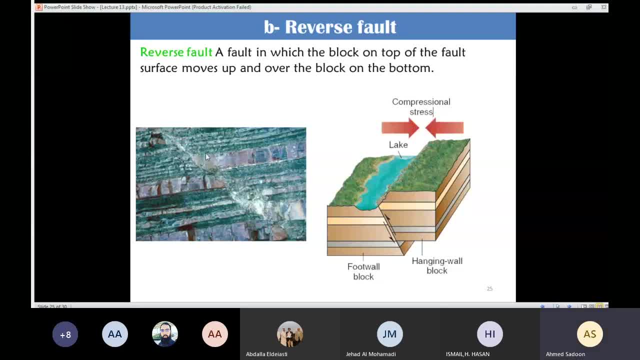 But this one Moved up Relative to that one, So in this case We are witnessing Reverse fault. I'm going to have to Transfer these two To the other side of the wall, So this one Is going to. 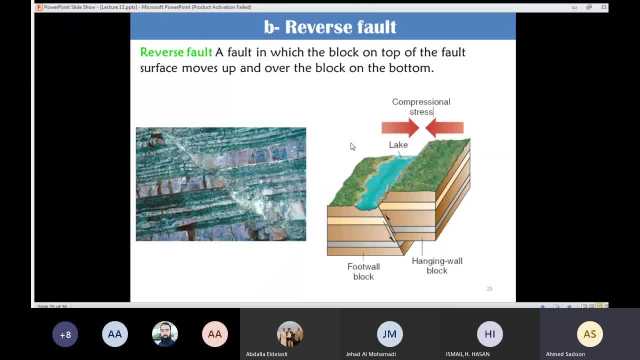 Move Out of the way. In that case The hanging wall Is going to move up And this one Is going to Move up. So this one Moving up material will affect the angle of the fault. no, it has nothing to do with. 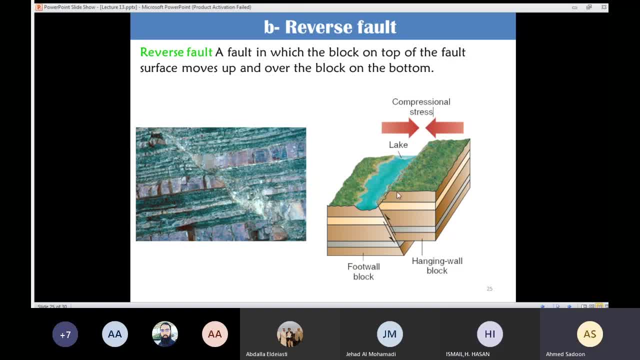 that nothing to do with the type of the material, unless you are talking about if it's ductile or if it's brittle. of course, for all of these cases the material it should be ductile or brittle for the fault to take place. it should be brittle because we, if you remember we are, when we were discussing about the 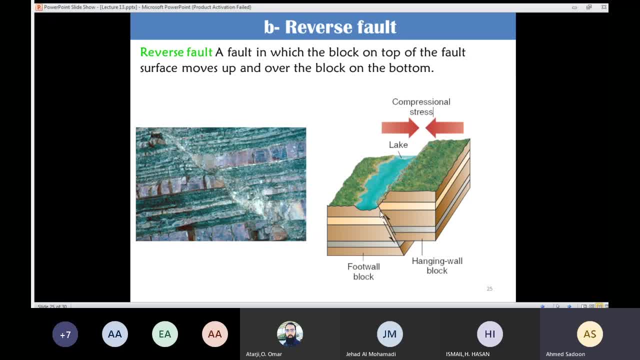 brittle behavior, we are going to have a sudden failure like this one. the material was the tile, then I'm going to have folding or stretching. so if I'm going to have a fault that means the material is brittle in the first point, then I'm going to have a fault that means the material is brittle in the first point. 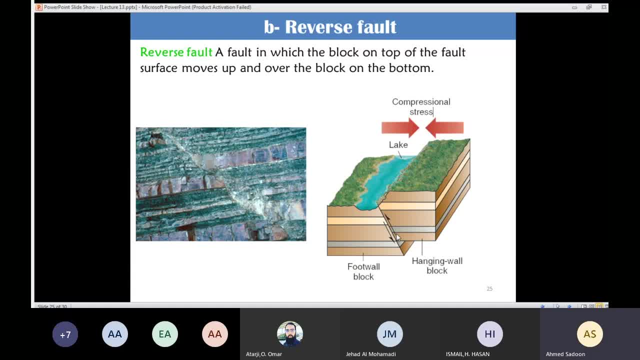 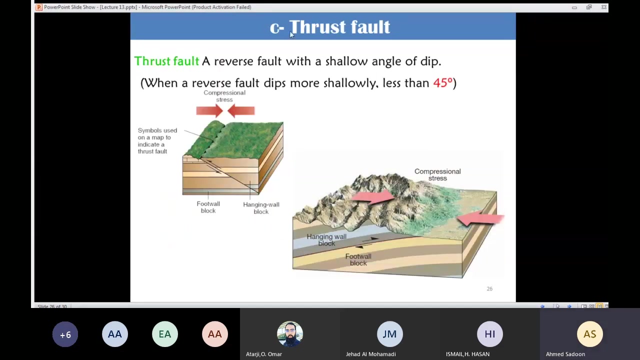 place. so I need to have condition. first condition: in order to have fault, the material should be brittle. the material is not brittle, in that case we are not going to have a fault. we are going to have a folder. okay, clear doctor. any other questions here? okay, let's move on. we have as a type which is a threat fault- this one is in- is. 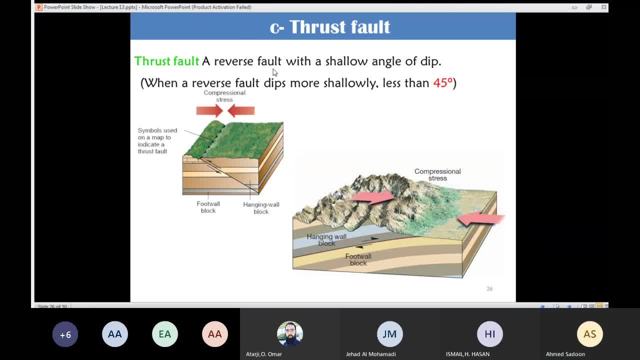 a special condition of the reverse fault, but in that case the angle of inclination is small, shallow, normally is going to be less than 45 degree. so the angle of inclination is small, shallow, normally is going to be less than 45 degree. so the angle here should be less than 45. 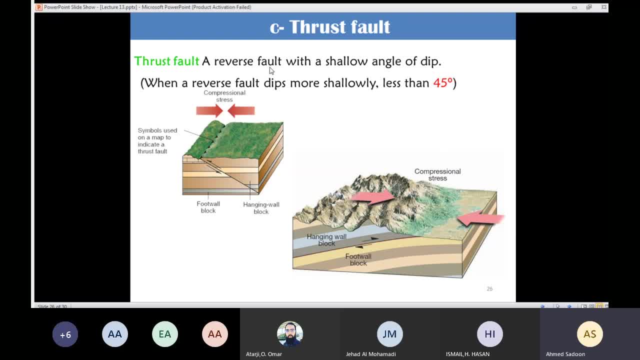 angle here should be less than 45 degree. so if I'm going to have reverse fault degree, so if I'm going to have reverse fault, which means that I have compressional, which means that I have compressional stresses and the hang wall is going to stresses and the hang wall is going to move up relative to the foot wall block, 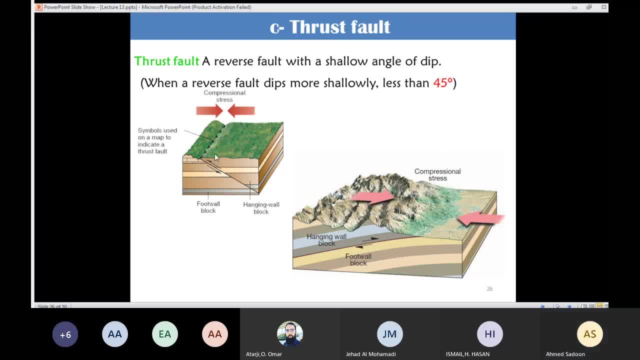 move up relative to the foot wall block. but here we have a special condition: the. but here we have a special condition: the angle of inclination is less than 45. angle of inclination is less than 45 degree. or it's very, very shallow in that degree, or it's very, very shallow. in that case, we are going to call the fault. 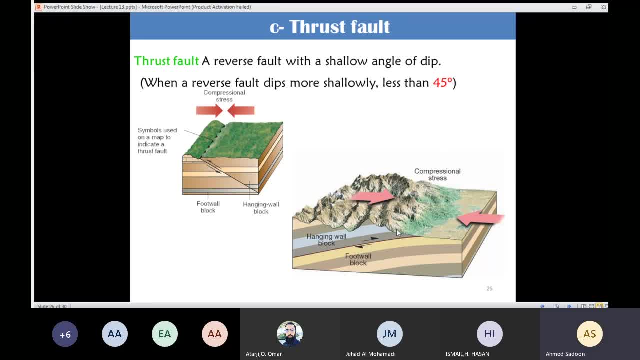 case we are going to call the fault thrust fault, like you can see here, the thrust fault. like you can see here, the angle of inclination is very small and angle of inclination is very small and the hanging wall is moving up relative. the hanging wall is moving up relative to the foot wall block and I have 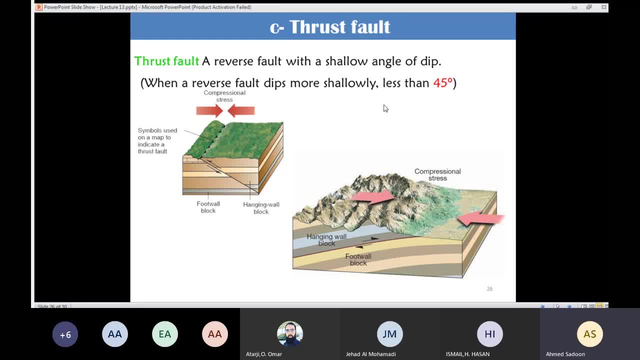 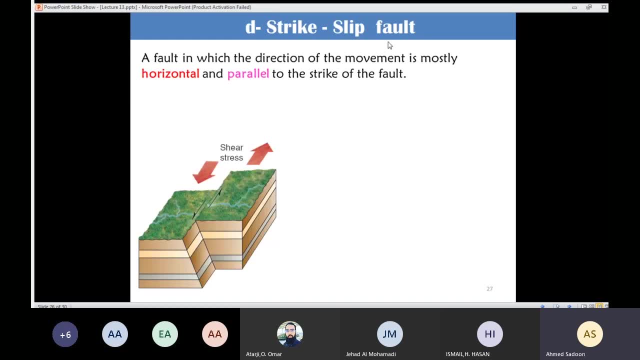 to the foot wall block and I have compressional stresses. so in that case, compressional stresses, so in that case I'm going to call it thrust fault. now I'm going to call it thrust fault. now we are going to move to different type of. we are going to move to different type of fault. 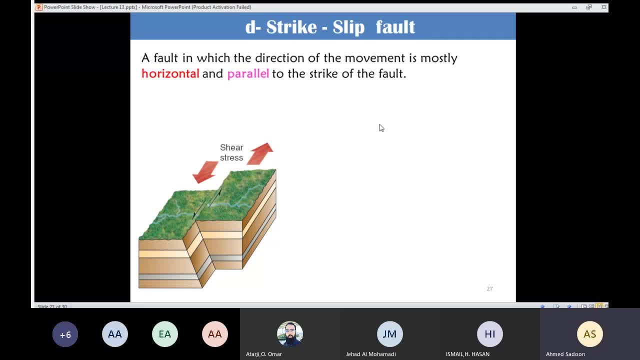 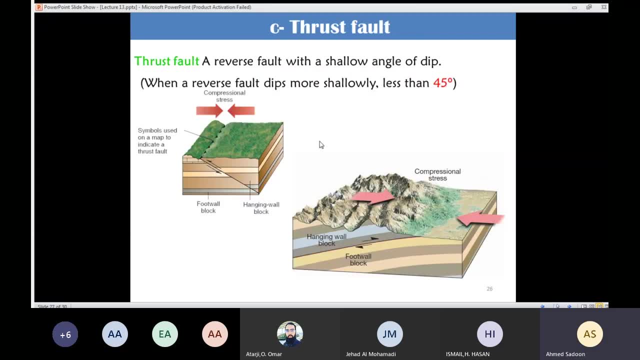 we are going to move to different type of fault. this time we are going to describe. this time we are going to describe this time. we are going to describe the fault by their strike. remember the, the fault by their strike. remember the, the fault by their strike. remember the strike here. said that in the beginning. 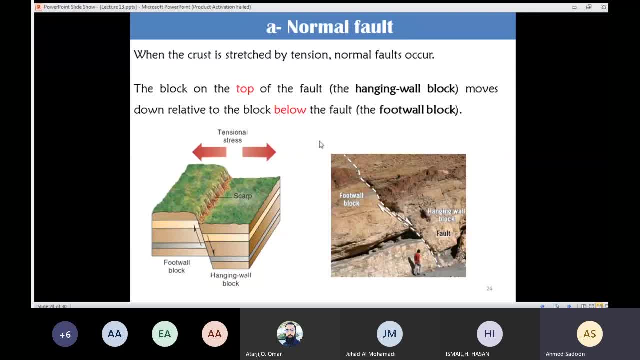 strike here said that in the beginning. strike here said that in the beginning we are going to describe the fault by. we are going to describe the fault by. we are going to describe the fault by their strike or by their dip- okay the, their strike or by their dip- okay the. 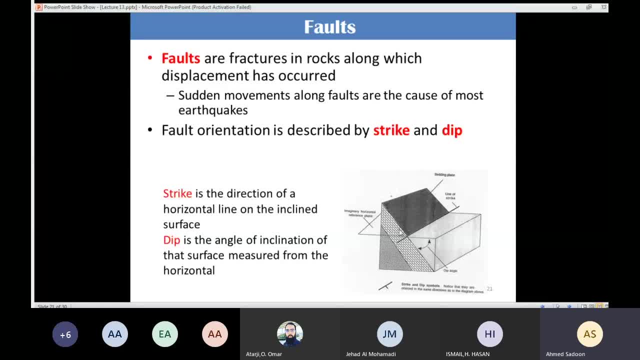 their strike or by their dip. okay, the strike is the direction of the strike, is the direction of the strike, is the direction of the horizontal line on the incline surface, this horizontal line on the incline surface, this horizontal line on the incline surface, this direction here and the direction here. 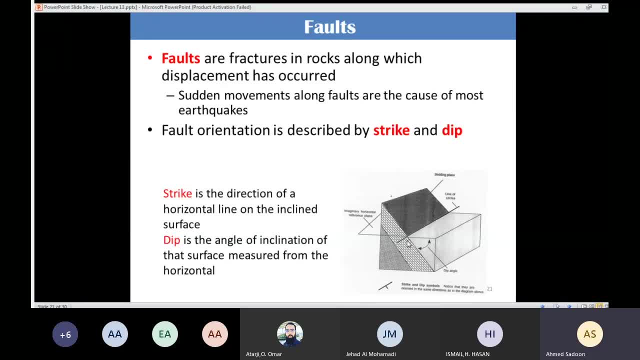 direction here and the direction here, direction here and the direction here, the direction, the direction here and the direction here, the direction of the dip. so the here, the direction of the dip, so the here, the direction of the dip. so the displacement it could move in that displacement, it could move in that. 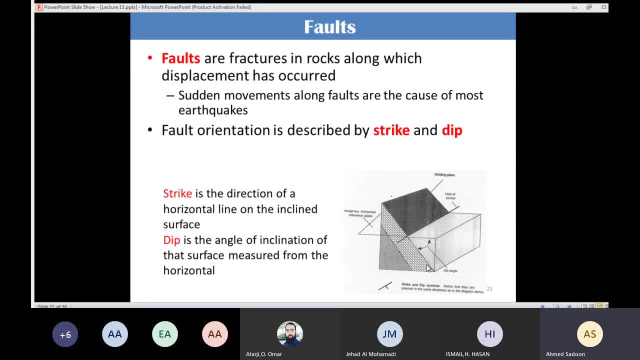 displacement. it could move in that direction or in that direction, the direction or in that direction, the direction or in that direction. the normal, the reverse the threats, all of normal, the reverse the threats, all of normal, the reverse the threats. all of them were moving in that direction here. 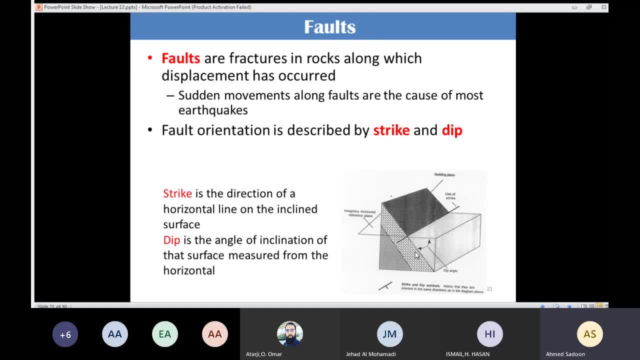 them were moving in that direction. here them were moving in that direction. here now for going to this the scribe. the now for going to this the scribe, the now for going to this the scribe. the fault by their strike. the displacement is fault by their strike, the displacement is. 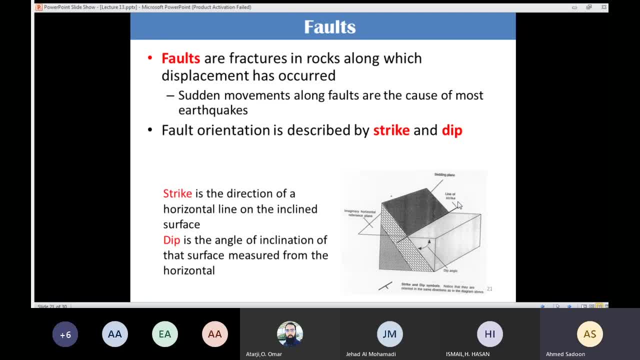 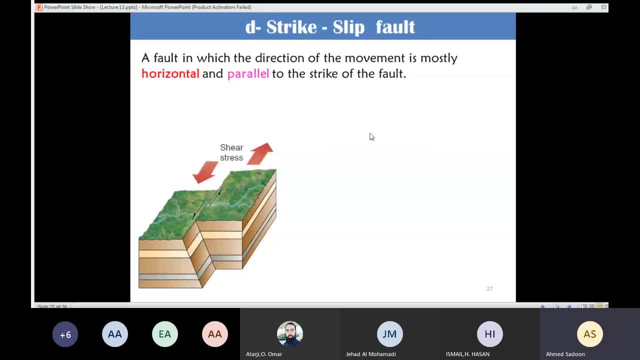 so let's get back here. we're going to talk about the strike slip. slip means talk about the strike slip. slip means talk about the strike slip. slip means displacement. strike slip means I'm going displacement. strike slip means I'm going displacement. strike slip means I'm going to have displacement in the direction of. 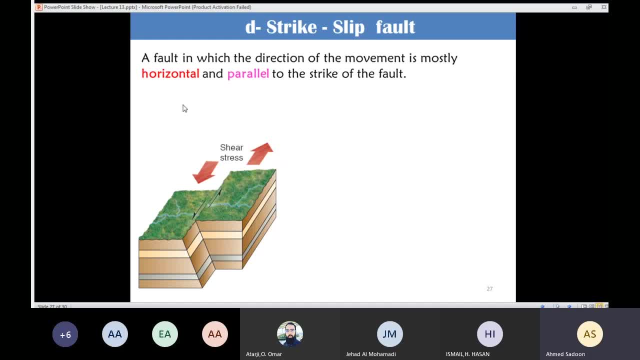 to have displacement in the direction of, to have displacement in the direction of the strike, so that case described by a, the strike. so that case described by a the strike. so that case described by a fault in which direction of the movement, fault in which direction of the movement. 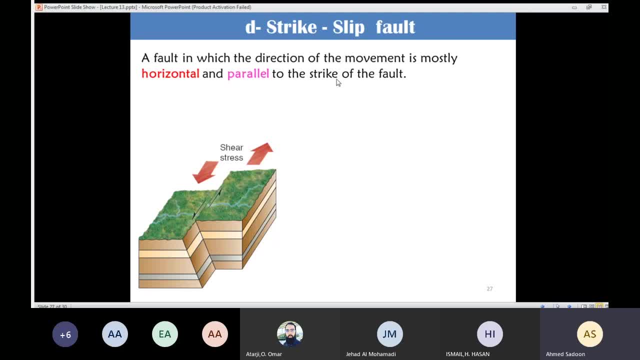 fault in which direction of the movement is mostly horizontal and parallel to the is mostly horizontal and parallel to the is mostly horizontal and parallel to the strike of the fault. so this one is strike of the fault, so this one is strike of the fault. so this one is direction of the dip and this one is the. 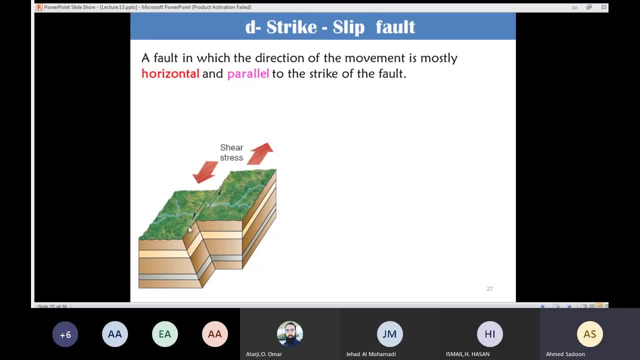 direction of the dip, and this one is the direction of the dip and this one is the direction of the strike. and, in case of direction of the strike, and in case of direction of the strike, and in case of strike slip fault as you might have, strike slip fault as you might have. 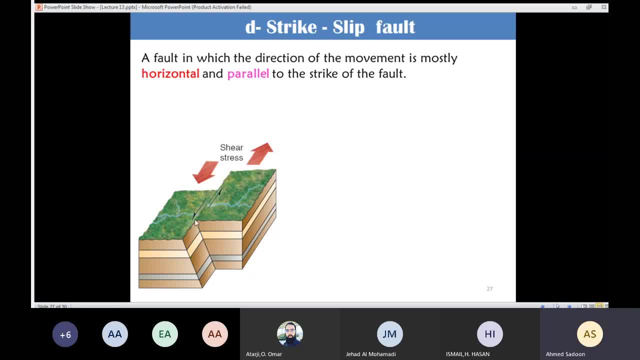 strike slip fault, as you might have guessed it. the movement is going to be guessed it, the movement is going to be guessed it. the movement is going to be in the strike direction, not in the dip in the strike direction, not in the dip, in the strike direction, not in the dip direction. so if I have that area here, 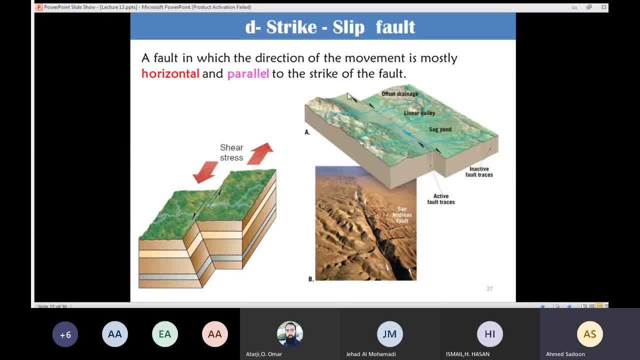 direction. so if I have that area here, direction, so if I have that area here, this part is going to move in that this part is going to move, in that this part is going to move in that direction, which which is parallel to the direction, which which is parallel to the. 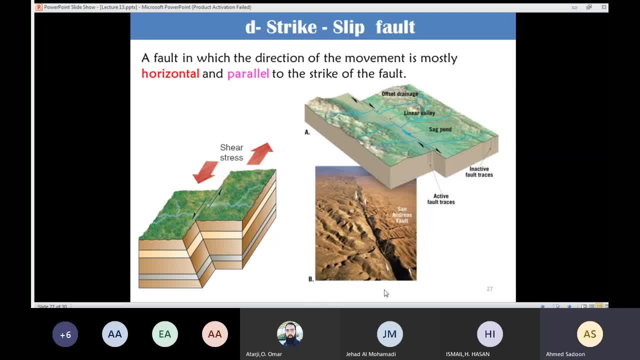 direction, which which is parallel to the strike direction, and this one is the strike direction and this one is the strike direction, and this one is the real picture for that in San Andres fault. real picture for that in San Andres fault. real picture for that in San Andres fault. I guess this one is in California. 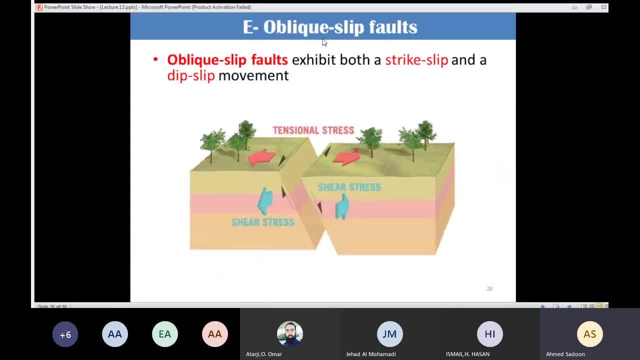 I guess this one is in California. I guess this one is in California. the last type of default is oblique slip. the last type of default is oblique slip. the last type of default is oblique slip. fault. this one is very special because fault. this one is very special because. 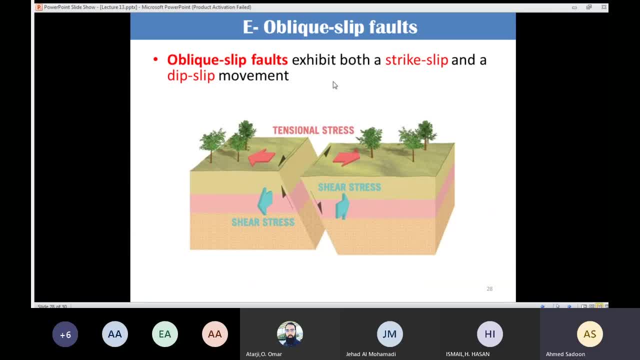 fault. this one is very special because this one exhibit or show both cases. you, this one exhibit or show both cases. you, this one exhibit or show both cases. you are going to have displacement in the, are going to have displacement in the, are going to have displacement in the strike direction and also are going to. 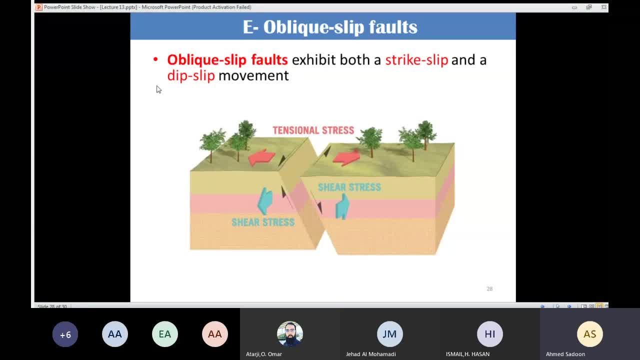 strike direction and also are going to strike direction and also are going to have displacement in the dip direction, have displacement in the dip direction, have displacement in the dip direction, so in the strike direction, here going to, so in the strike direction, here going to, so in the strike direction, here going to have displacement, and in the dip. 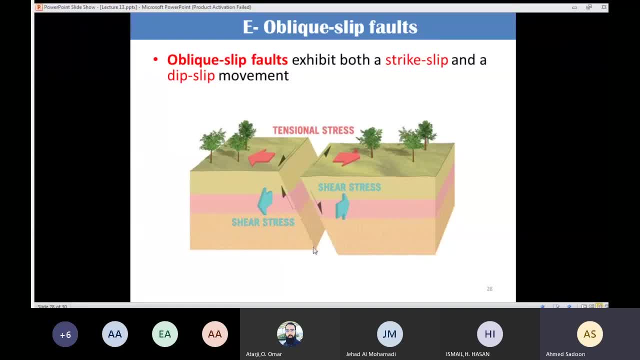 have displacement and in the dip have displacement and in the dip direction, here I'm going to have direction, here I'm going to have direction, here I'm going to have displacement, and if that case is displacement, and if that case is displacement, and if that case is presented, we are going to call it. 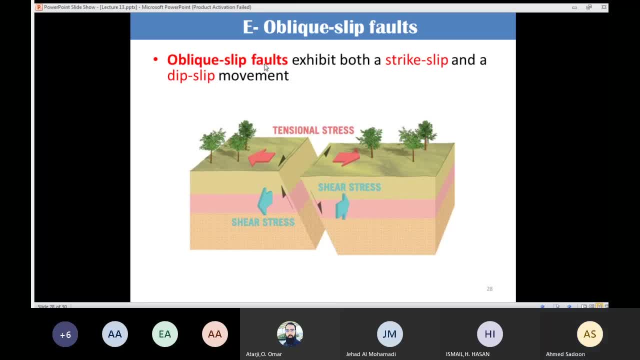 presented. we are going to call it presented. we are going to call it oblique slip faults. so I need to have oblique slip faults. so I need to have oblique slip faults. so I need to have tension on stresses. I'm going to tension on stresses, I'm going to 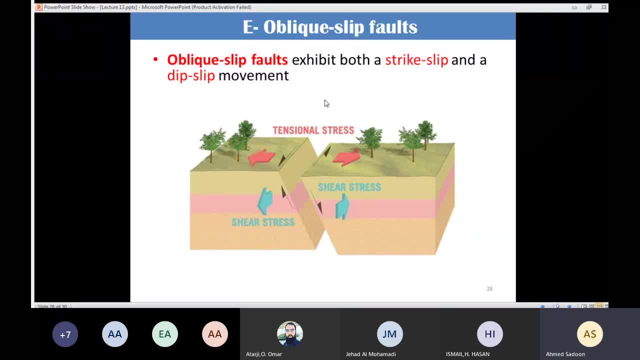 tension on stresses. I'm going to witness displacement in witness, displacement in witness, displacement in the strike direction. I'm going to witness the strike direction. I'm going to witness the strike direction. I'm going to witness displacement in the dip direction. so displacement in the dip direction. so 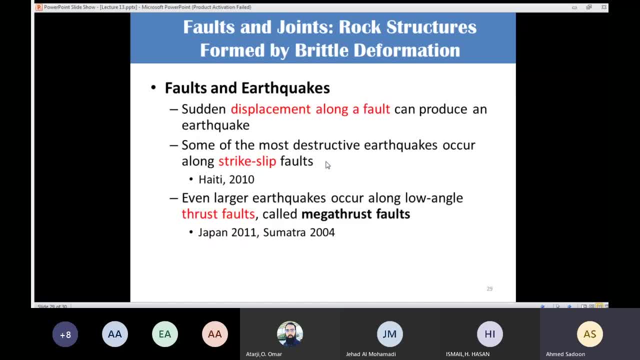 displacement in the dip direction. so this one is very dangerous and in the, this one is very dangerous and in the, this one is very dangerous. and in the beginning I said that defaults is beginning. I said that defaults is beginning. I said that defaults is associated with the earthquake, the 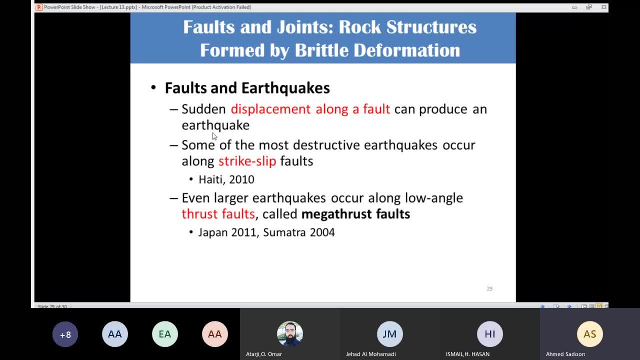 associated with the earthquake. the associated with the earthquake. the sudden displacement along the fault can sudden displacement along the fault can. sudden displacement along the fault can produce an earthquake. some of the most produce an earthquake. some of the most produce an earthquake. some of the most destructive earthquake occur along strike. 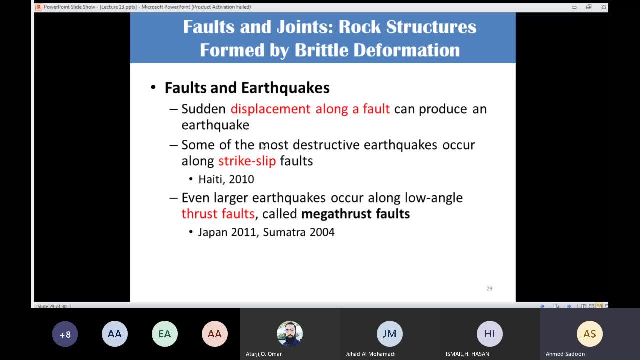 destructive earthquake occur along strike. destructive earthquake occur along strike slip slip displacement along the strike direction, And something like that took place in Haiti in 2010.. And even larger earthquakes occur along low angle thrust fault. If the angle is very low, we are going to call this mega thrust fault. 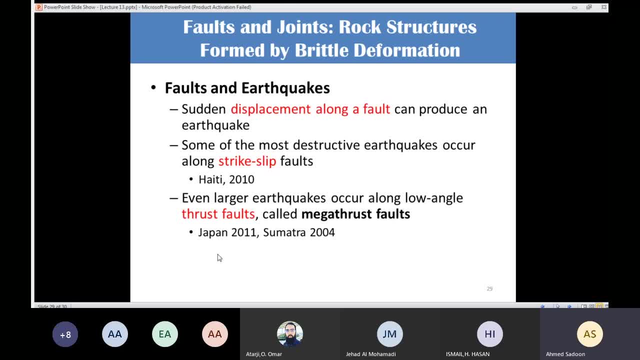 An earthquake like this one took place in Japan 2011 and in Samarta 2004.. And if I do remember that, I think catastrophe take place there in Fukushima nuclear plant And I think the city is still locked up today. So earthquake it could be very dangerous. 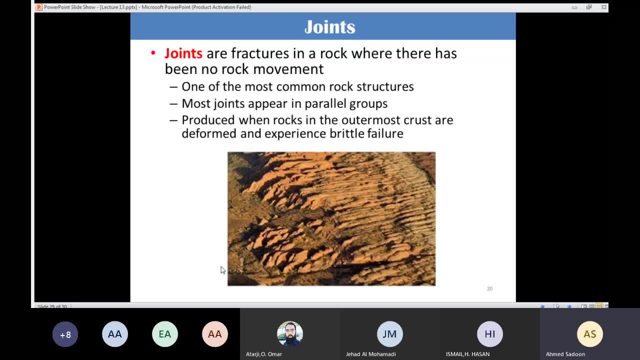 The last thing Which I want to talk about is the joints. The joint is very simple. They are going to have fractures in the rock, but without displacement, Not like the faults, And most joints appear in parallel groups like this one. They are going to be parallels and in group. 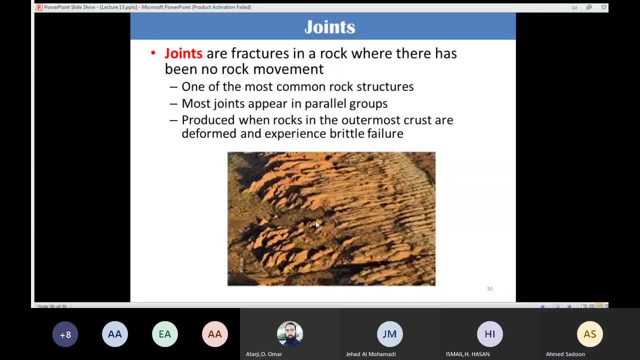 And, of course, without displacement. And it's one of the most common rock structures And produced when rocks in the outermost crust are deformed And experience brittle failure. So joints are very simple. You are going to have fractures and it's going to be presented in the outermost crust. 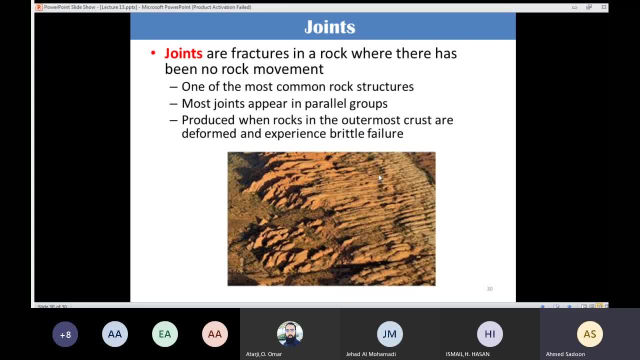 And the behavior should be brittle And they are going to be parallel to each other. Now I'm done with the crustal deformation And I'm going to show you how it works. If you need, if you are interested or you need more information, you can get back to.